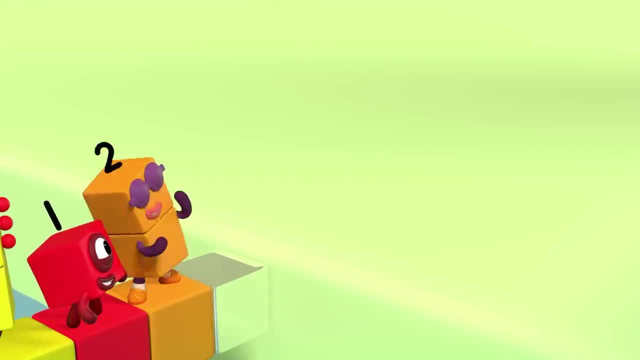 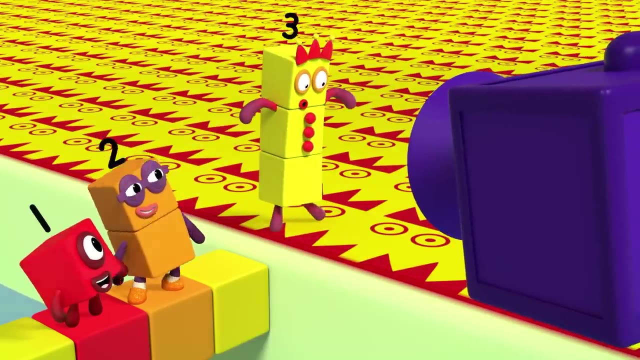 Tell me the pattern: Red, Orange, Yellow, Oh, Pattern unlocked. Ooh, Now, that's what I call a pattern. Ooh, Oh, I know exactly what to do here. so if you, uh, Green, green, green green, jump over the gap. 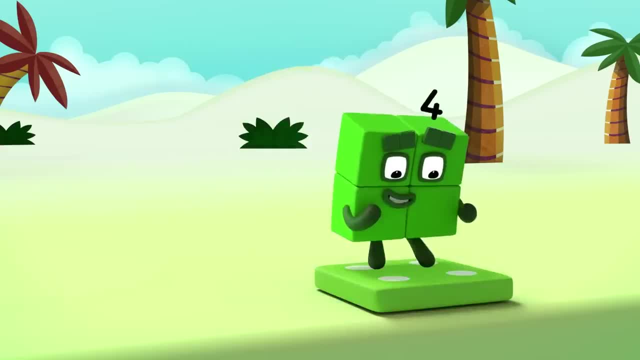 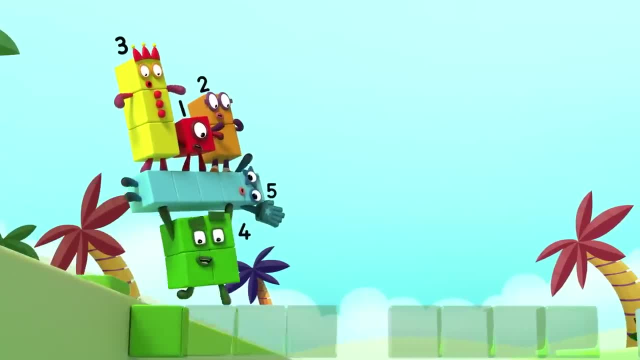 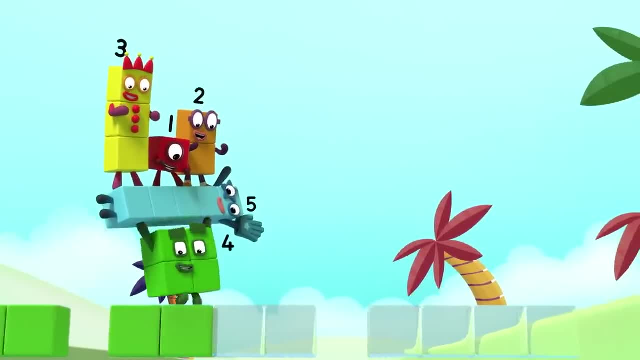 Green, green, green, green, jump over the gap. Ooh, Green, green, green, green, jump over the gap. Tell me the pattern. The pattern is it goes: four greens, then a gap and repeat. Pattern unlocked. 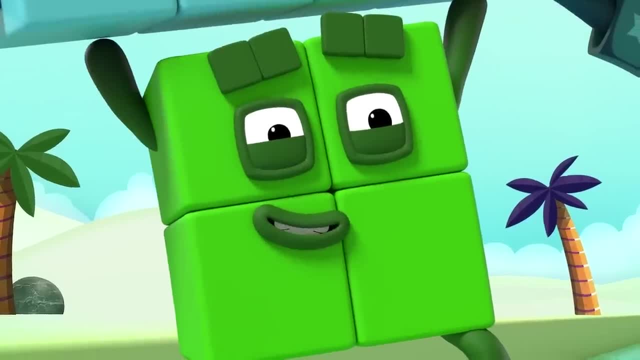 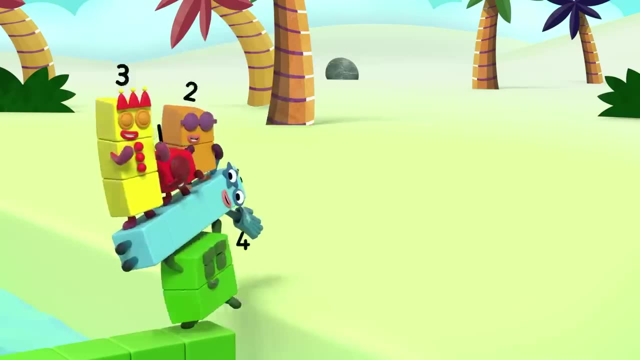 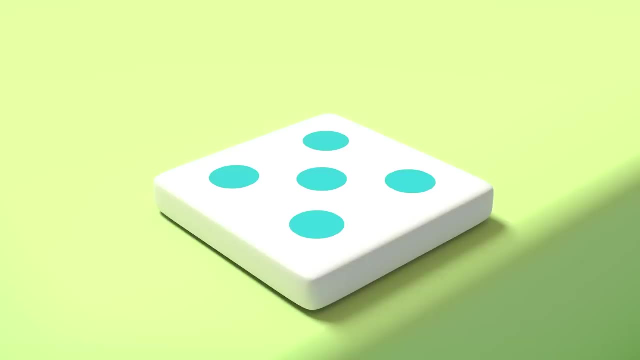 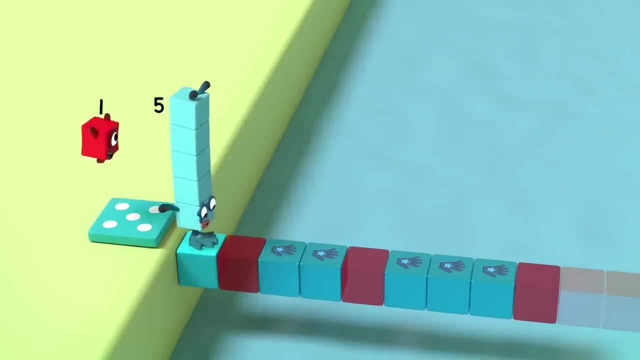 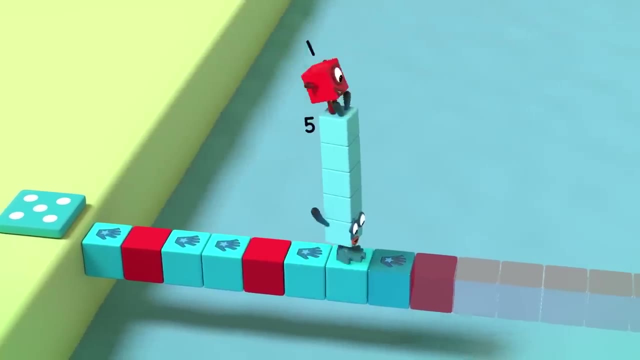 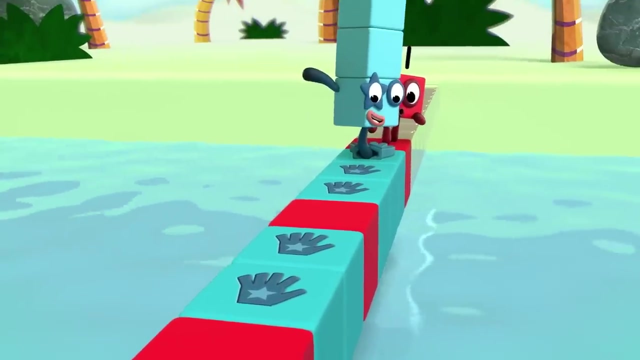 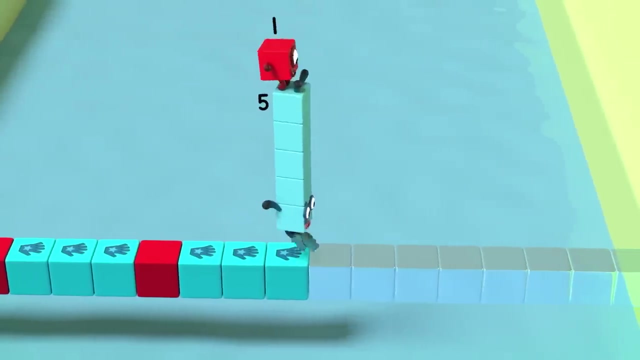 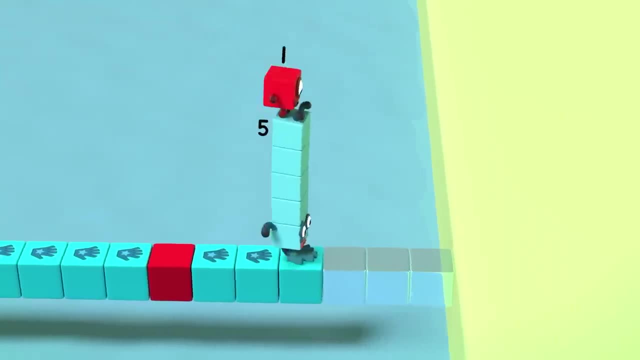 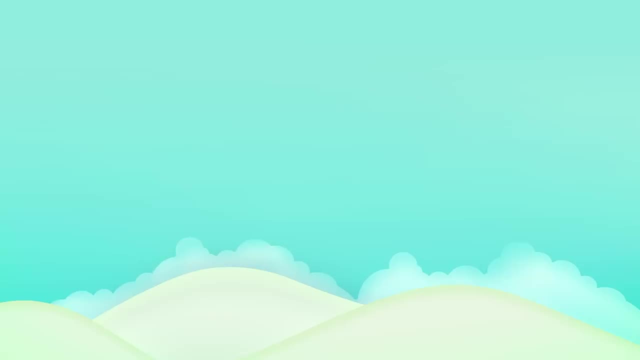 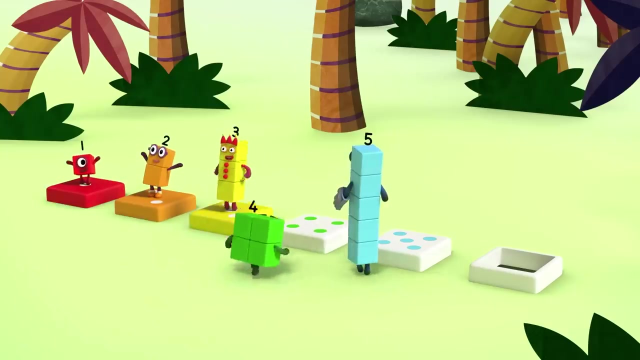 Oh, Oh, Oh, Oh Oh. Pattern unlocked. Look, we're at the centre. Oh yeah, One, two, three, four, five, six Pattern unlocked. You got across my pattern paths. Well done everyone. 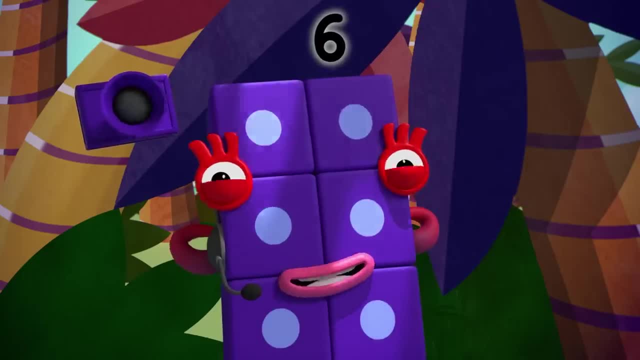 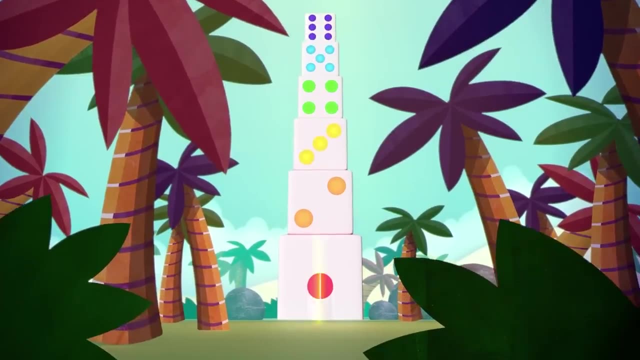 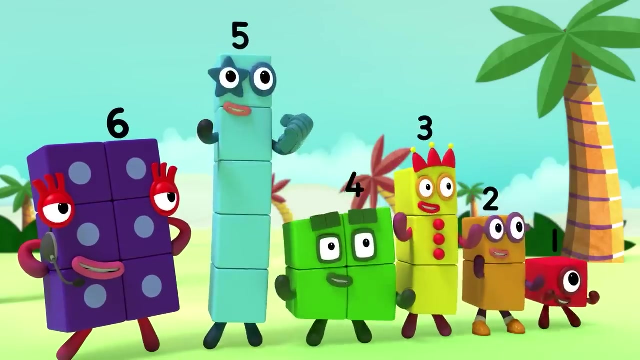 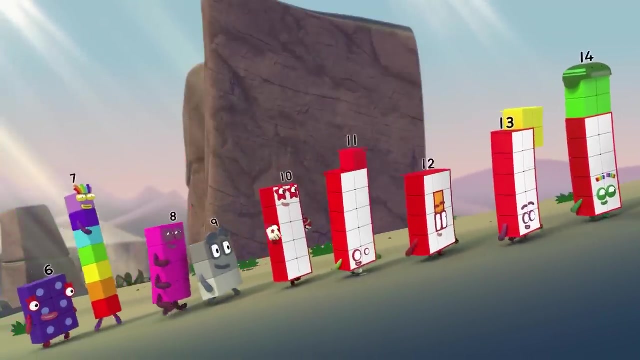 Now step into my pattern palace and let's all have some fun. Whoa, Pattern palace unlocked. I can't wait to visit the pattern palace. Is it far? There's a shortcut round this ridge if you can cross the balancing bridge, Wow. 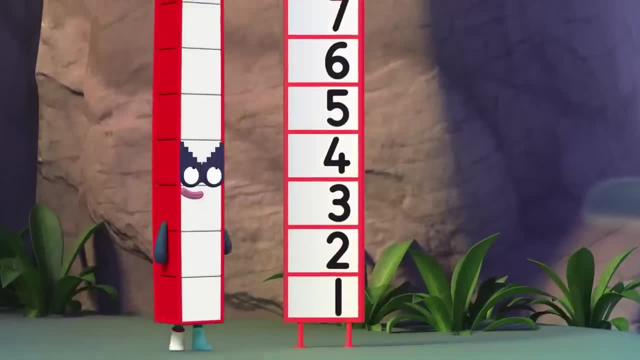 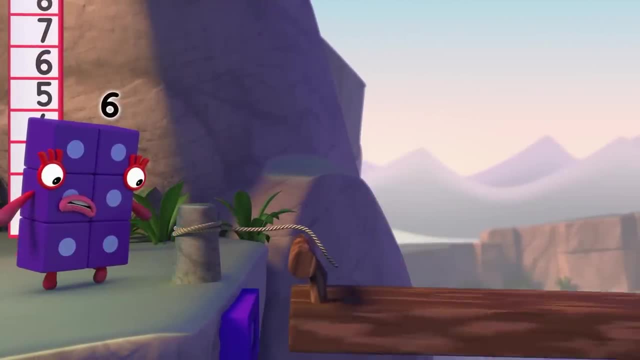 Oh look, it's the pattern palace. It's a little bit like a castle. It looks like a castle in a palace And it's got a wall and a pulpit at the front. One, two, three, four, five, six. 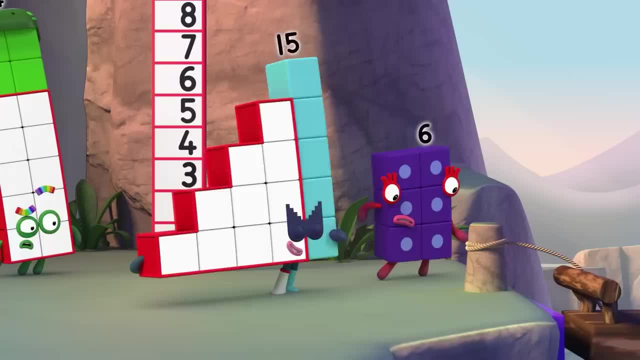 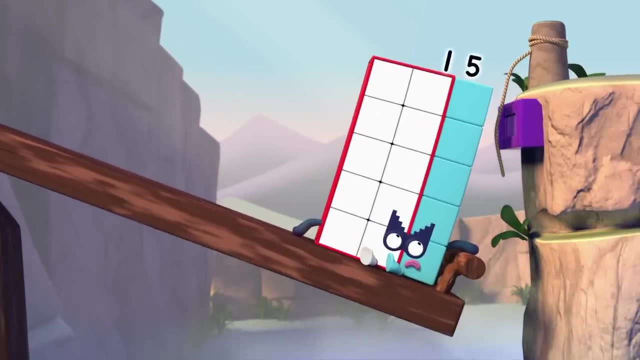 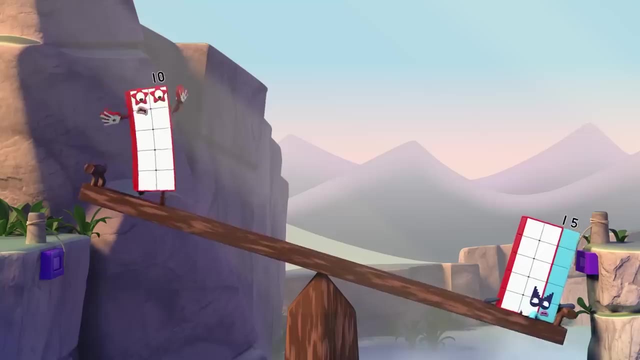 You've got to step into the pattern palace. We're at the pattern palace again. Let's go. I think it's time to take a look at the pattern palace. Ta-da Whoops, Guess I forgot to put the safety locks on. 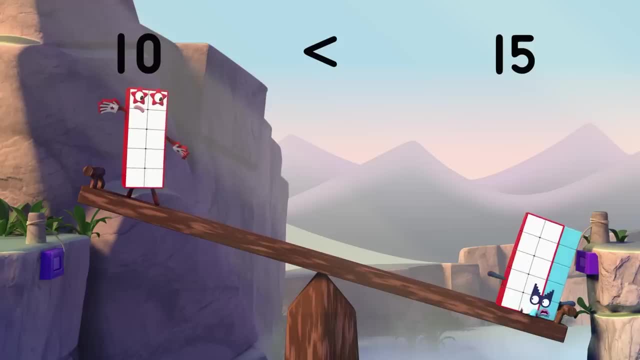 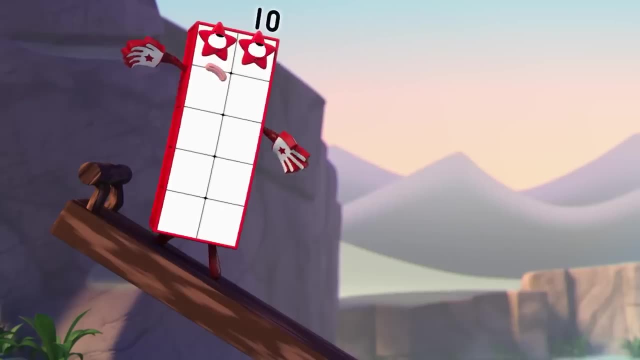 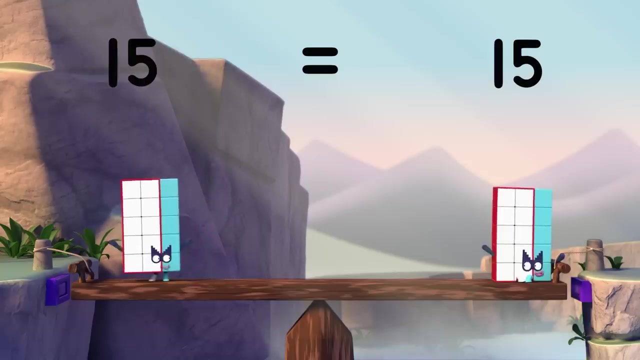 I say we go softly, softly, Fifteen. You need fifteen blocks to balance me out, But fifteen is ten and five, so if I land a hand, Two plus five equals fifteen. Grab hold. We need to reach the far side so we can lock the bridge. 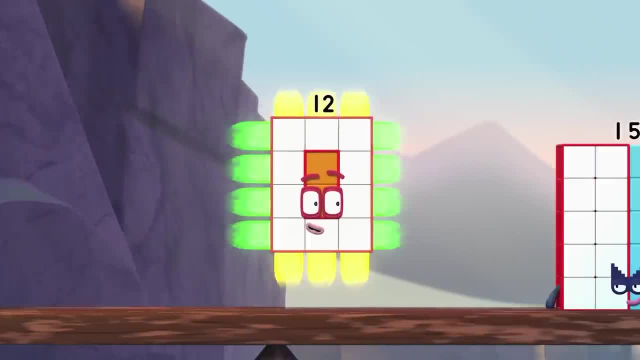 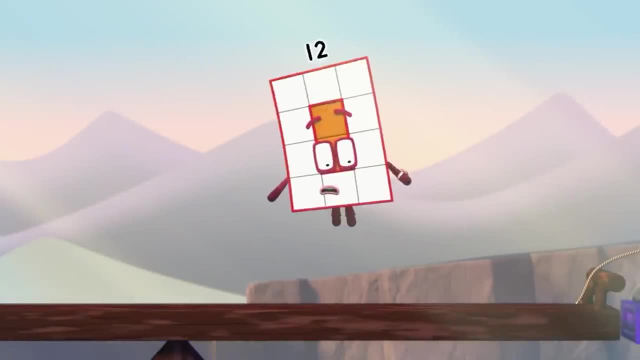 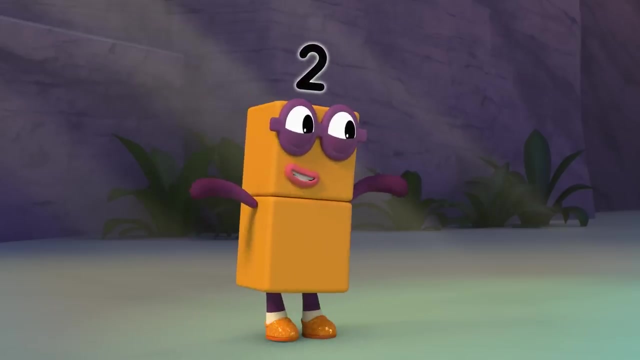 I can do this. I am three by four. I am a rectangle. Wow, That is so cool. Thanks, What's going on? Twelve needs balancing And twelve is ten plus two. Come on, ten. Wait, Where's ten? 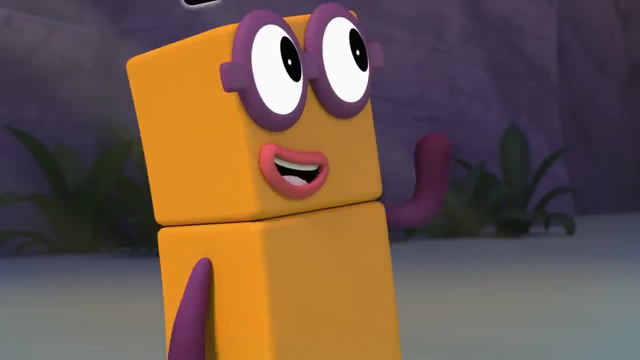 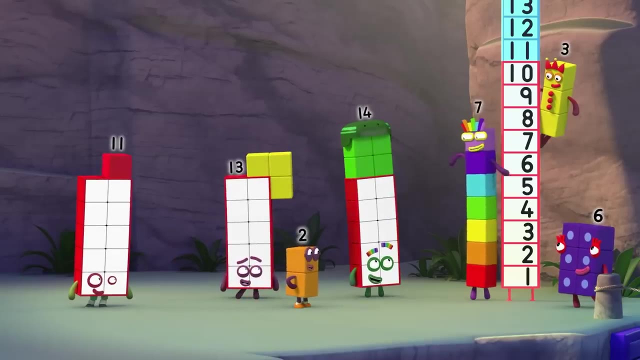 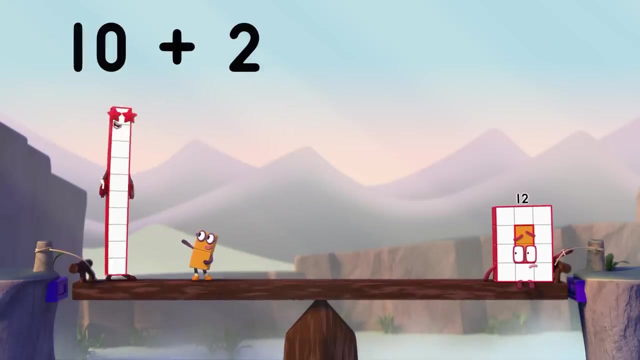 Bit busy, Sorry. Then we need another ten, Seven, three, You can make ten, That's lucky. Seven plus three plus two equals Ten plus two equals Twelve. Grab hold, Yay, We're halfway there. What could possibly go wrong? 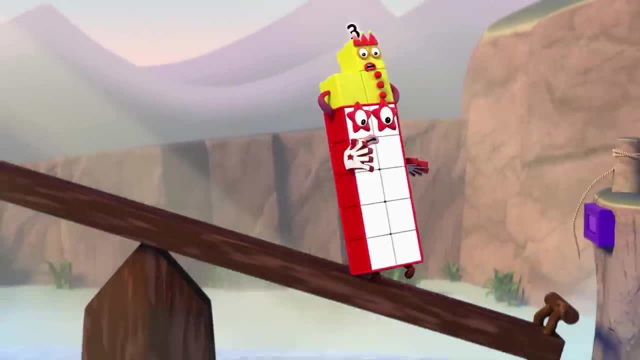 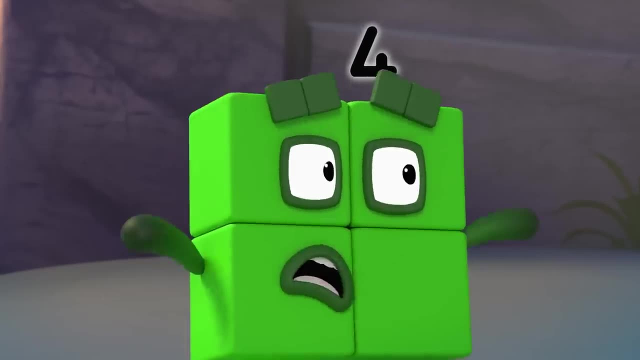 Ooh, Look out Thirteen. You said it. Oh, We need to balance Thirteen, But we haven't got a three Or a ten. Maybe I can help. I'm only one less than ten. That's close. 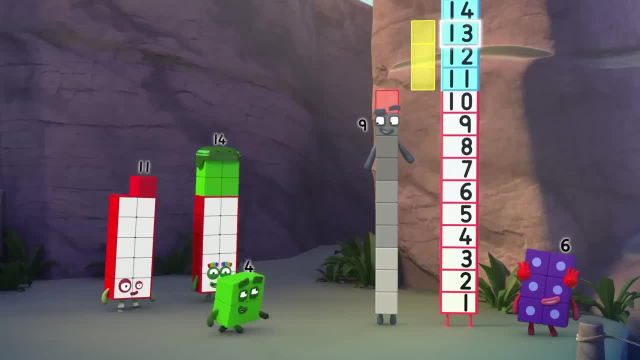 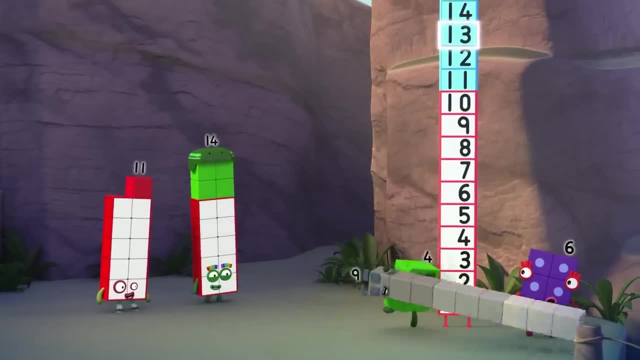 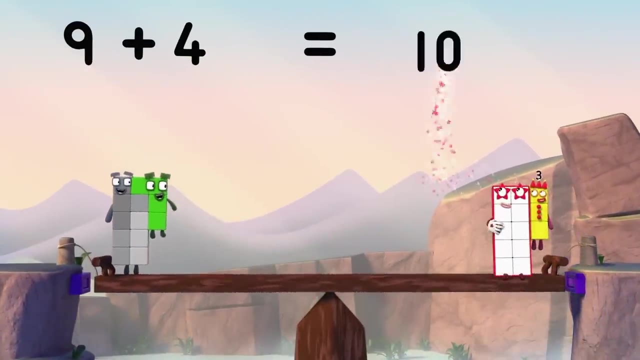 And after that we need three more blocks. So that adds up to One, two, three, four, Four blocks. Square power: Nine plus four equals Ten plus three, And both sides equal thirteen, Thirteen, Woo-hoo. 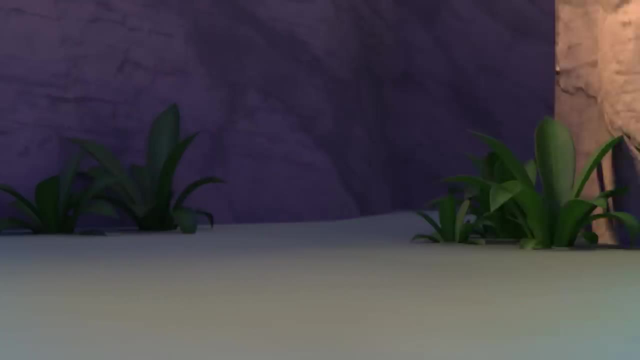 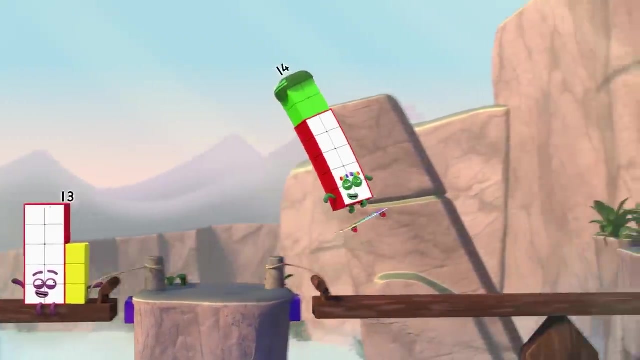 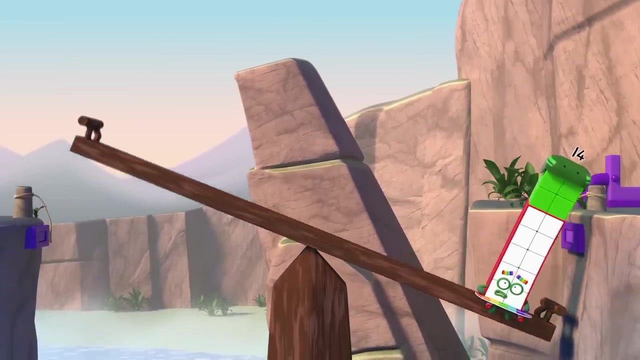 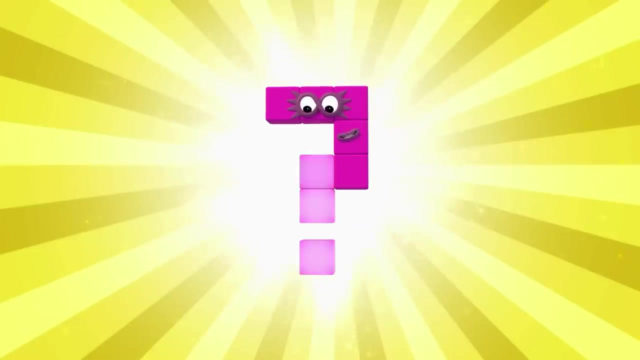 Grab. hold One more bridge to go. Woo-hoo, Hey-oh-oh, We need to balance out Thirteen Somehow. Octoblock think One, two, three, four, five, six, seven, eight. 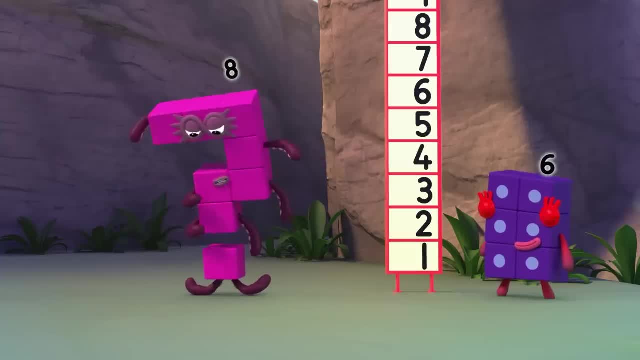 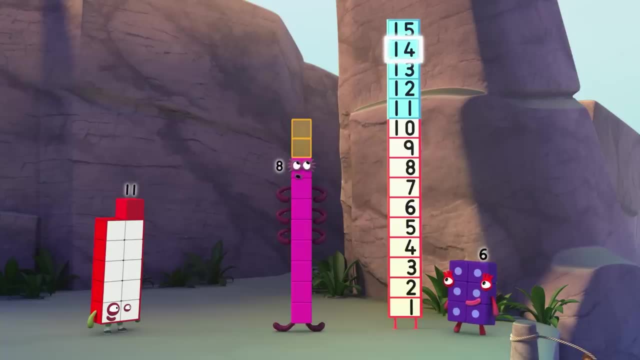 Think: Hmm, How do I get from eight to fourteen? Ha, From eight to ten takes two blocks, And fourteen is ten and four. So I need four blocks more, Which makes One, two, three, four, five, six. 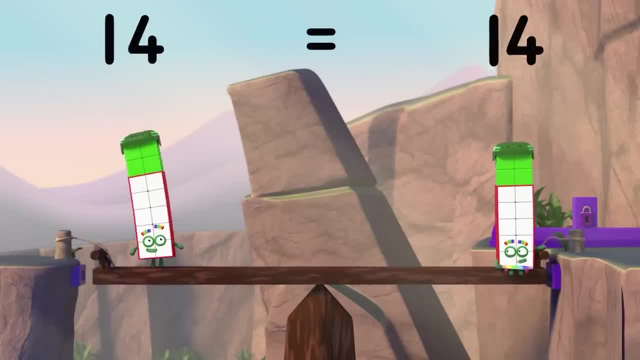 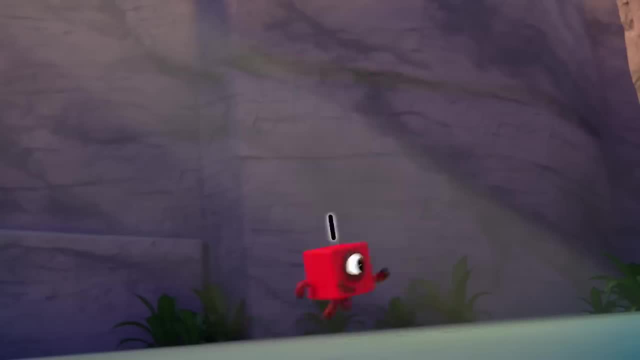 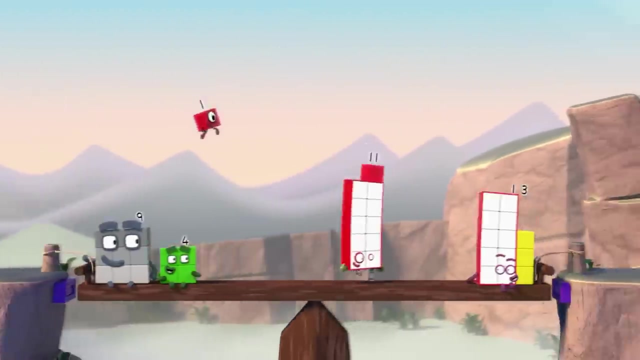 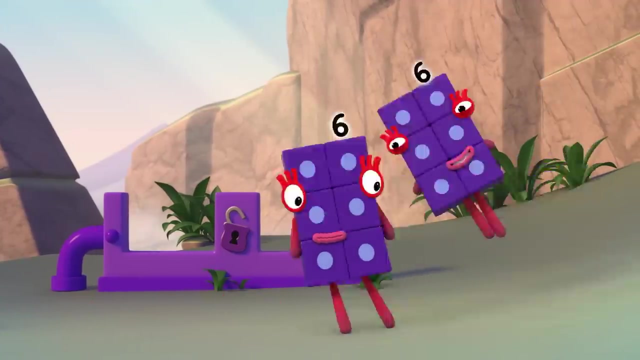 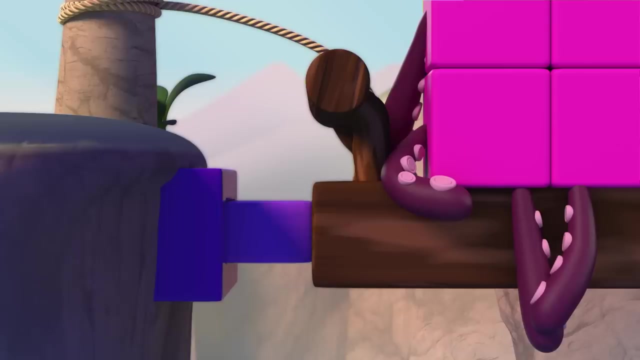 Eight Plus six Equals Fourteen Grab hold. Thanks to our team, We've got a clear run at goal. Double six Bridge is fixed. structural noise, Heave-ho, Wee-heave-ho Shit. 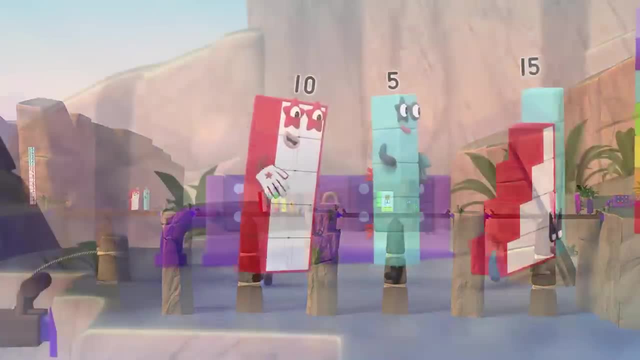 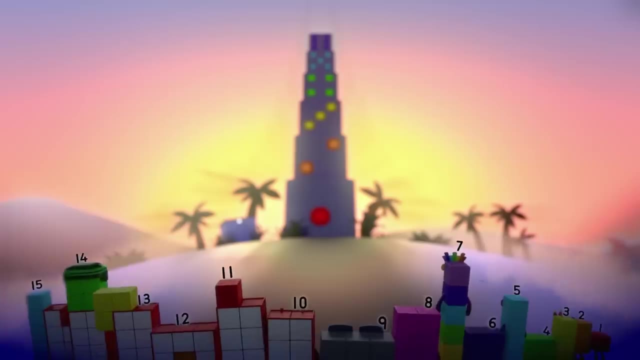 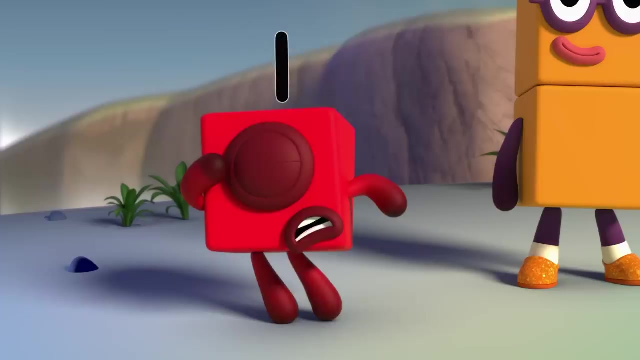 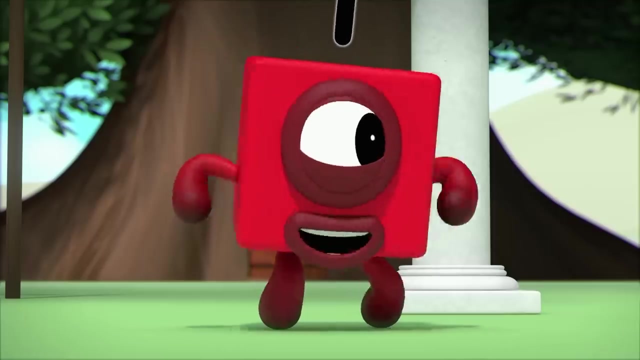 Hm, Hm, Hm, Hm, Hm, Hm. I guess this shortcut's not so swift. Next time we can take the lift. There's a lift Six Steps Squares. Is everyone ready for the annual Steps vs Squares treasure hunt? 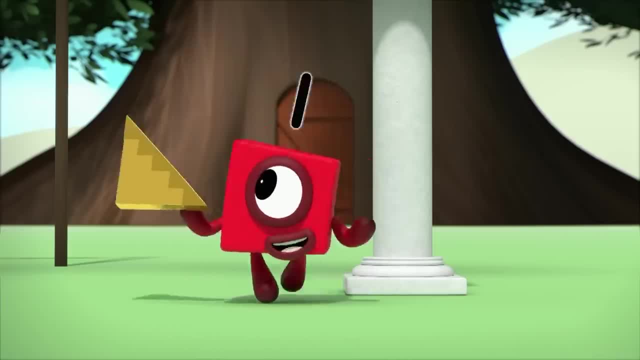 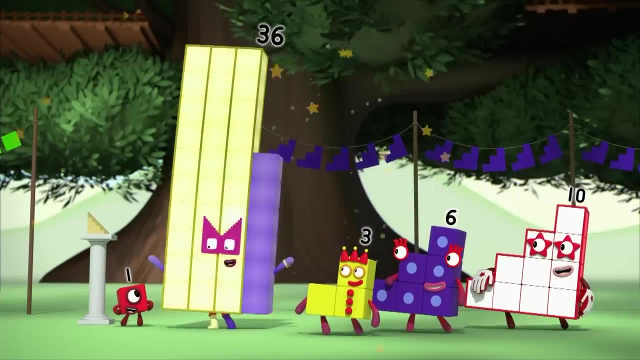 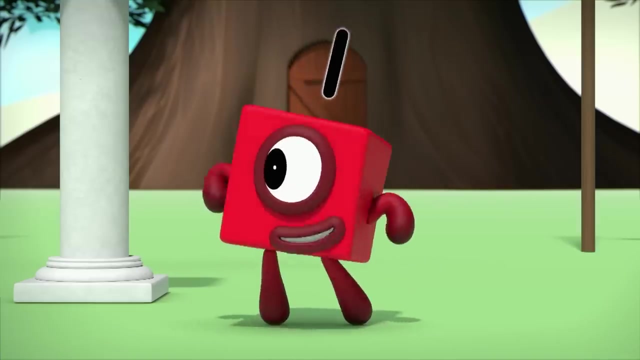 Whoever brings back the most trophy pieces wins. You can use any tricks and skills you like. Oh, sounds like fun. Don't mind me, I am 36 and I am a big fan of tricks. Then stick around and watch. Anything goes in this contest, Including starting, before I say go. 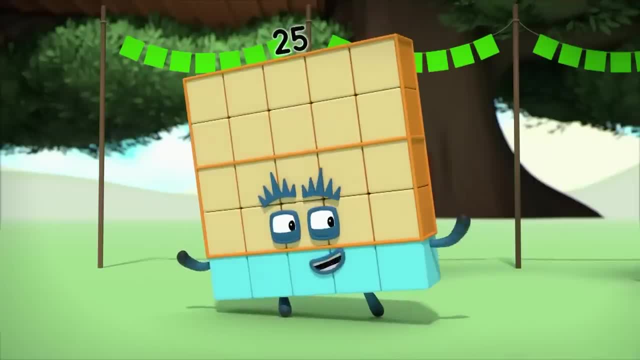 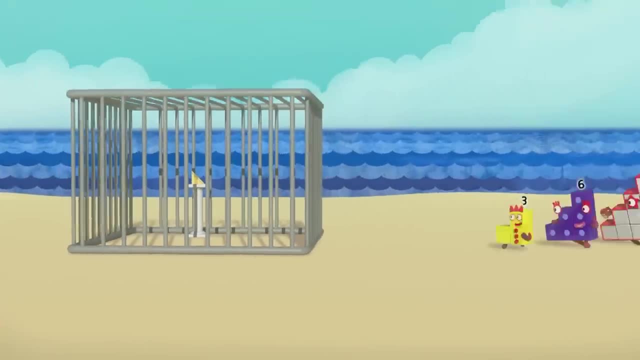 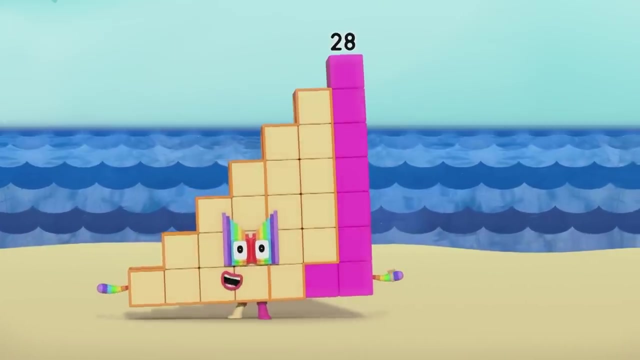 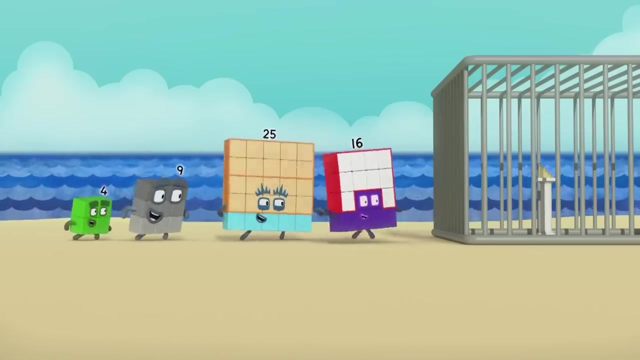 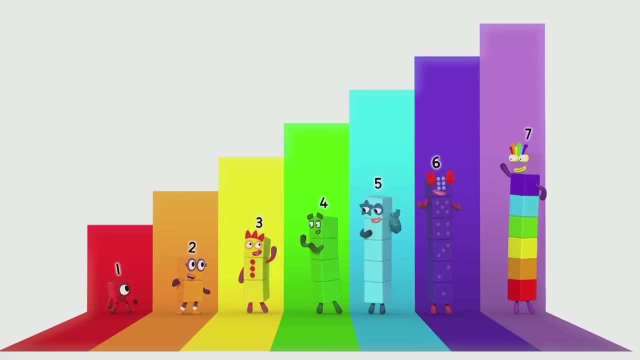 Looks like we're one step ahead. Hey, come on squares after them. There it is the next trophy piece. I have a perfect seven-step plan. Step one: Find a helicopter and fly it over the beach. Step two: Lower a rope towards the cage. Step three: 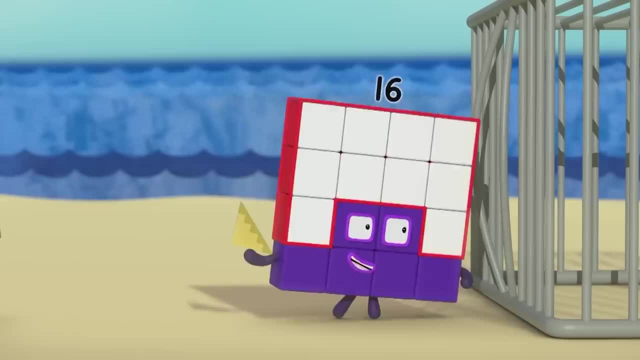 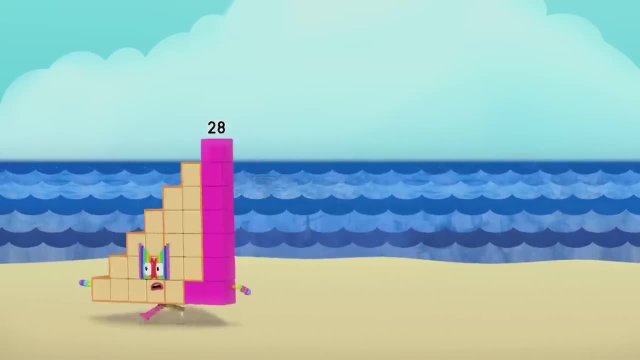 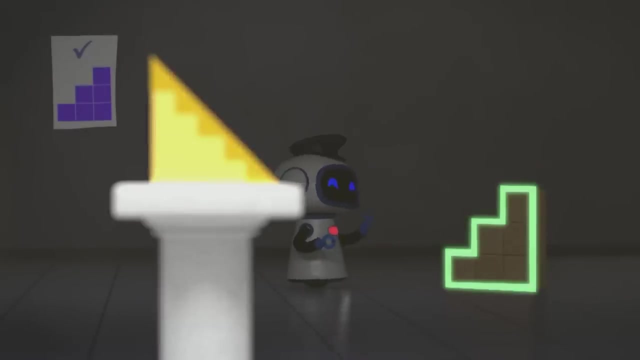 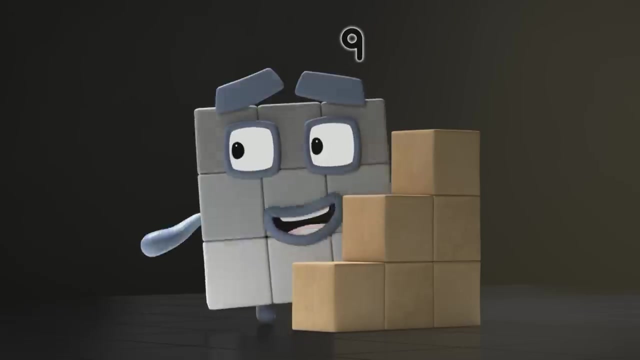 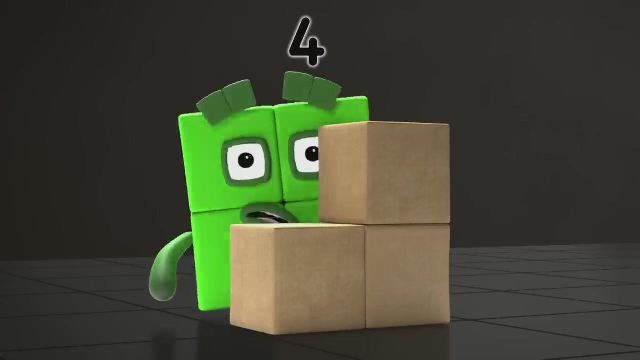 Tie a gigantic magnet to the. You snooze, you lose. Oh, After them. Step shape detected, all clear. Look there it is. How do we grab it without being spotted? Shame, we're not step-shaped. Quick hide four on the floor. 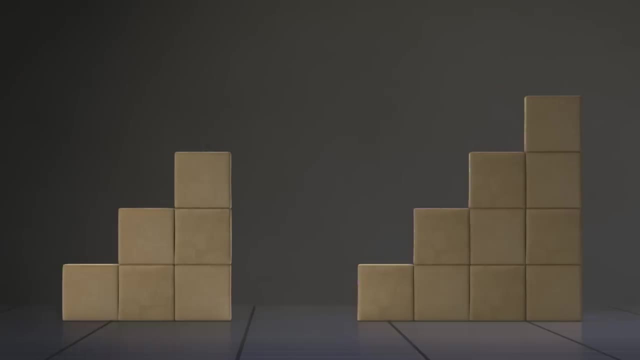 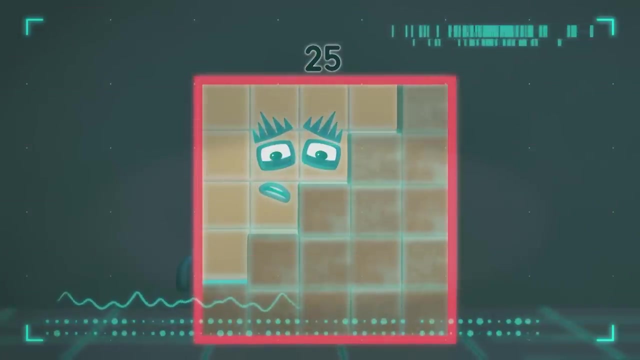 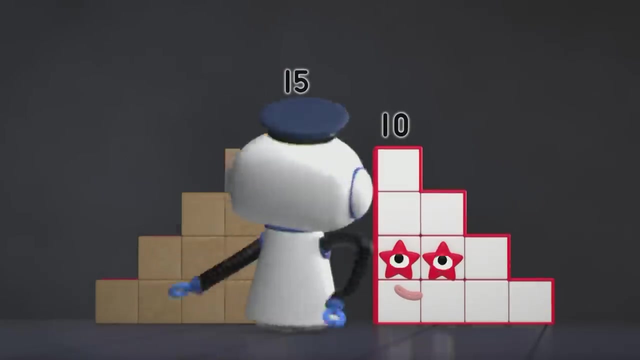 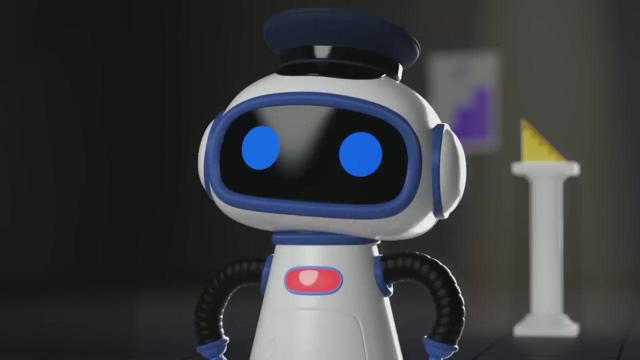 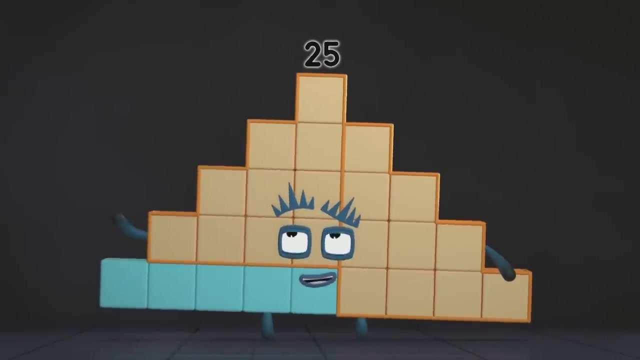 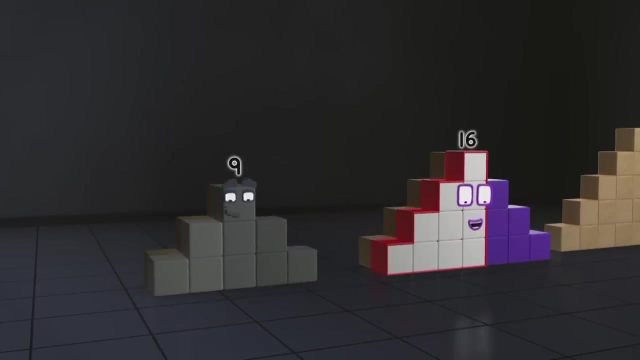 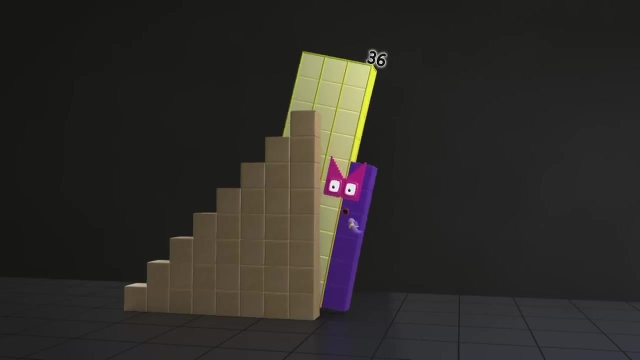 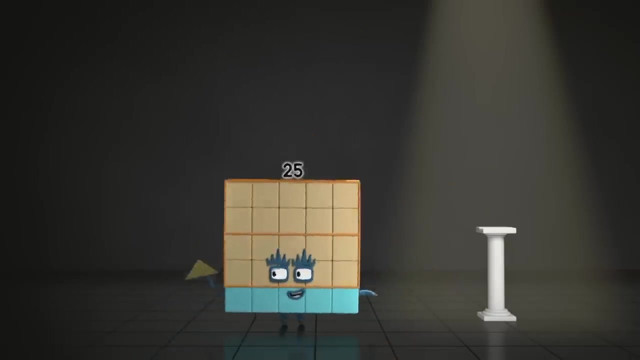 What, Oh, dear Alert. Non-step shape detected. Hush-hush, perfect camouflage Step shapes detected, all clear. Look at this: squares can make up-and-down steps. Huh, So we can Very tricky Beep, oop, Oh, Oh, Got it quick before it. 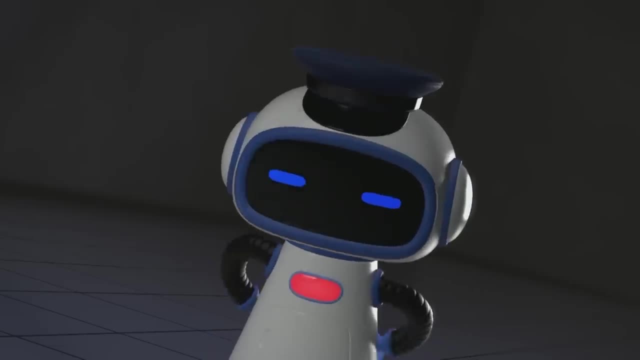 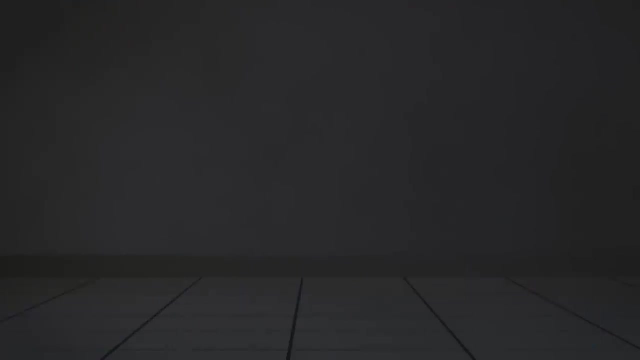 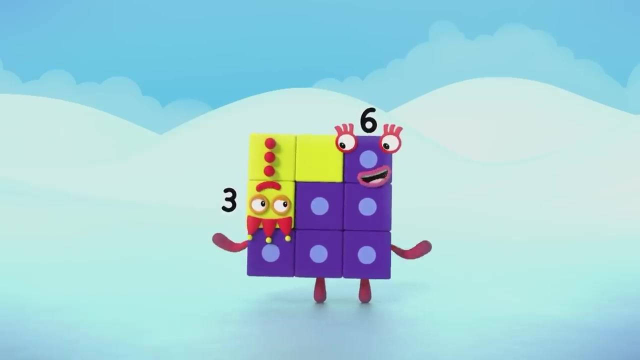 Entruder alert. Tickle, tickle, Tickle, tickle, Tickle, tickle, Run for it, Run for it. It's not fair. Those strong squares could break this ice like: Eh Whoa, I got you and look what we can do. 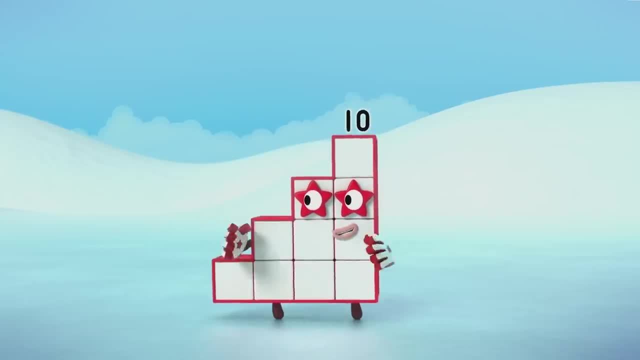 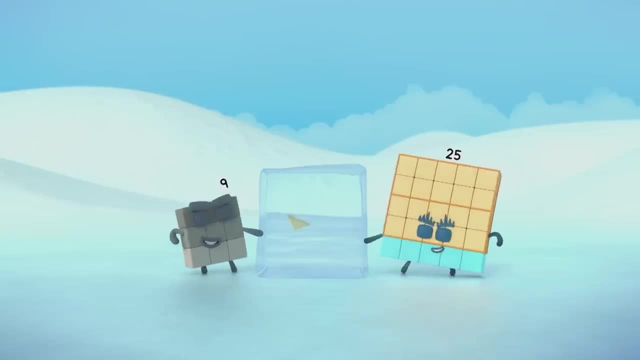 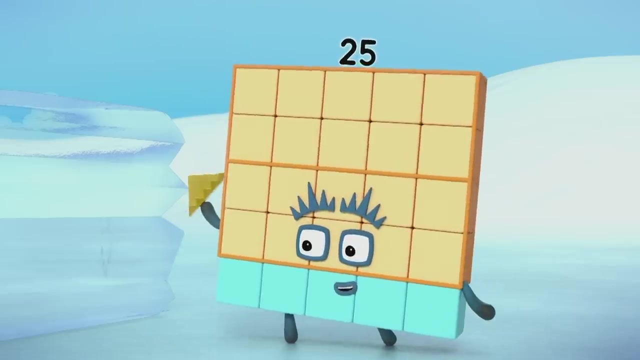 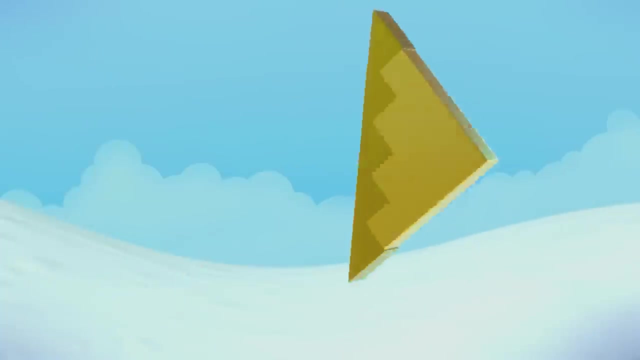 Ooh, Two step shapes can make a square. We can beat them at their own game. Hoop Oh, Hoop, Hoop, Hurray. Step Squads are the best. No, What happened there then? Welcome back. Let's count your pieces and see who's won. 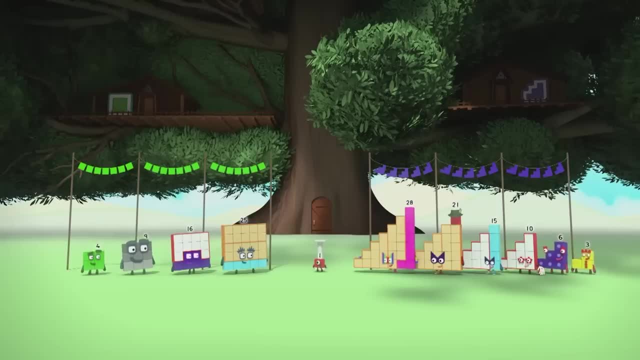 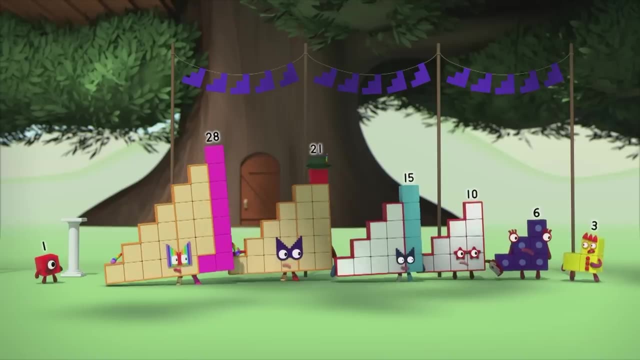 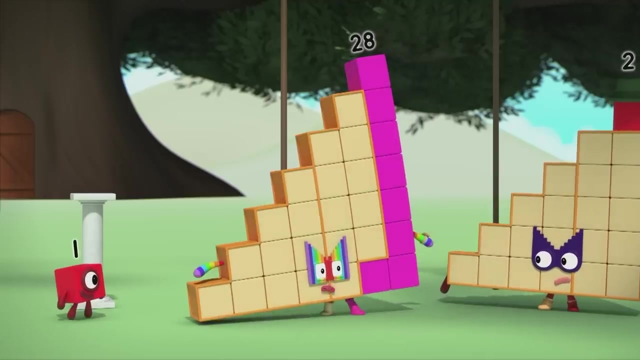 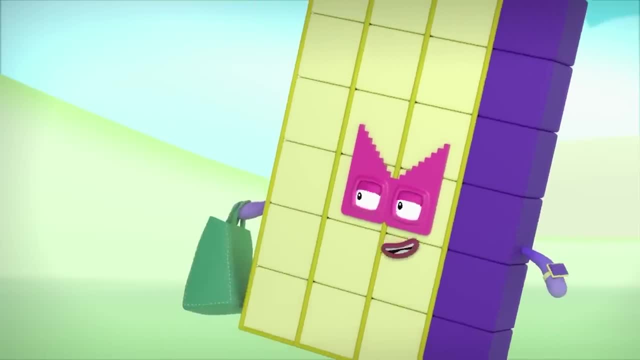 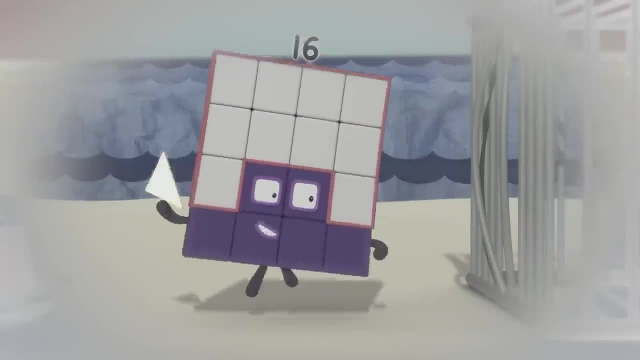 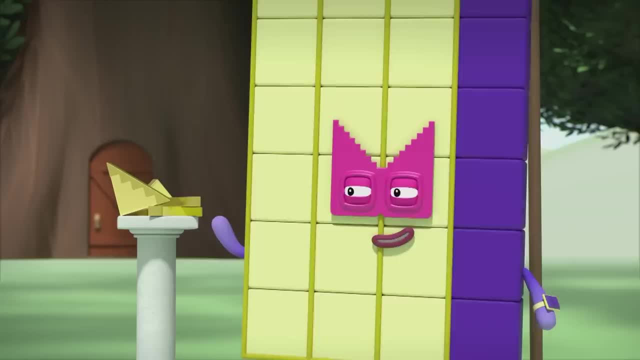 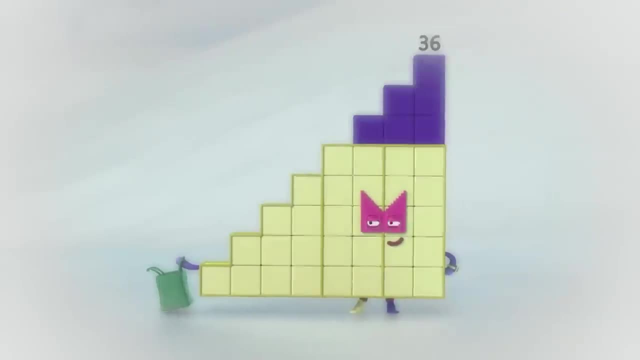 You gave me a trophy- piece 28,- when I was step-shaped, And you gave me the second piece 16, when I was square. Wait, are you a Stepsquad or a square? Yes, exactly, I mean, I'm both. 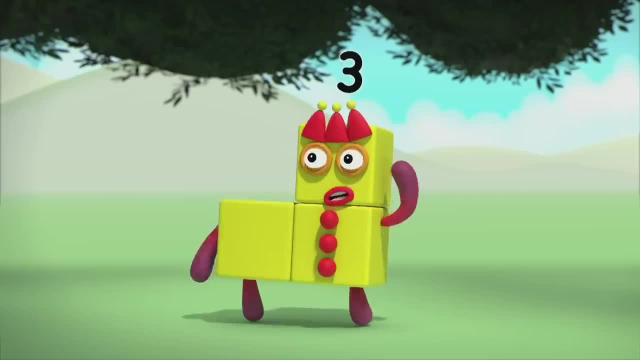 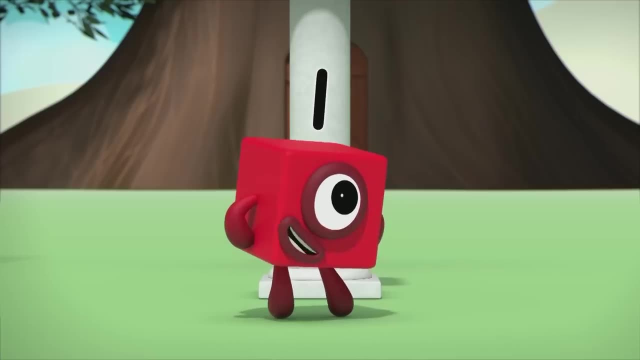 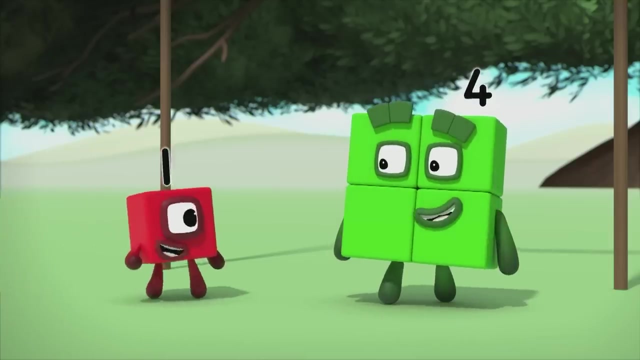 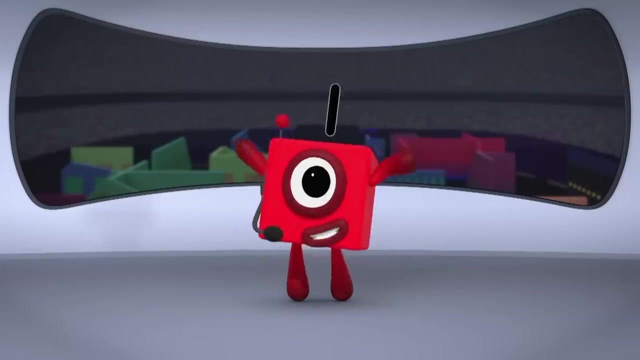 I am Puzzle Master 36.. But who won Steps or squares? That's easy, You both did, because 36 was on both teams, which is a nice trick if you can manage it. Welcome to the Team Tag-o-wina for another exciting game. 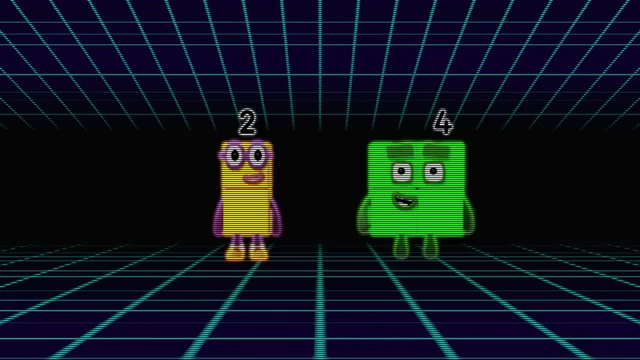 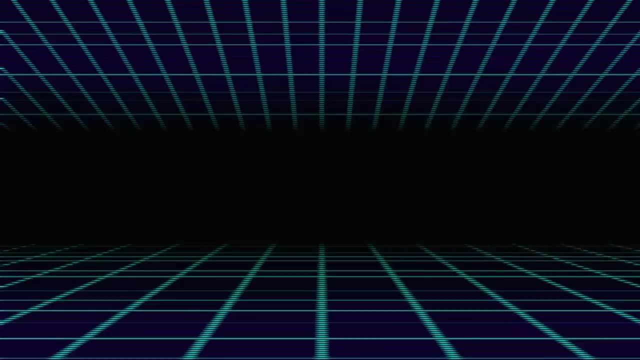 There's only one rule to Team Tag: If you tag someone team of twos and they can make a team of you, they join your team And we're off Big numbers first to give them a chance to run and hide. 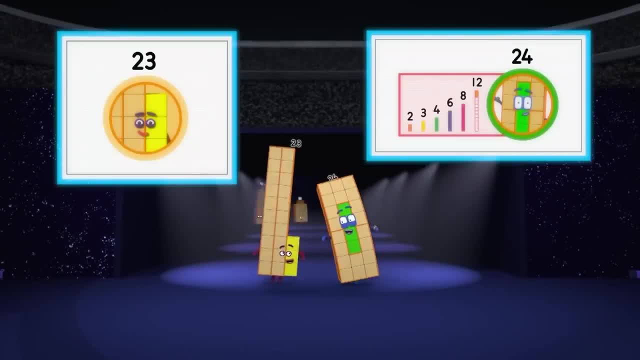 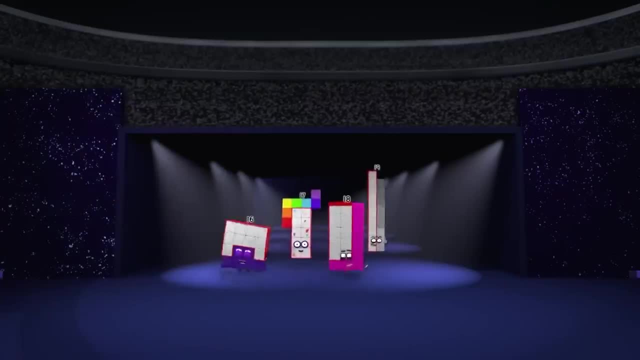 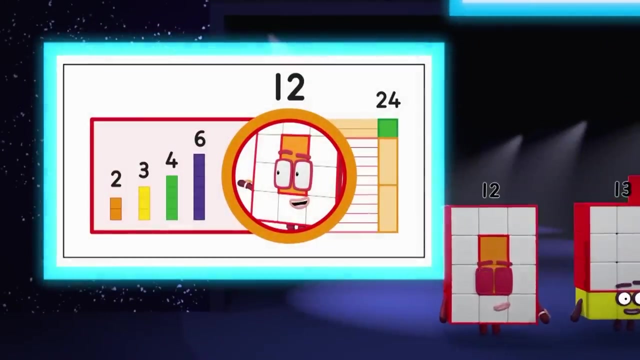 See how many different number blocks can tag 24.. The lower 20s next, And here come the teens. There's 12,, the first of the chasers looking to tag 24, but needs to stay away from 2,, 3,. 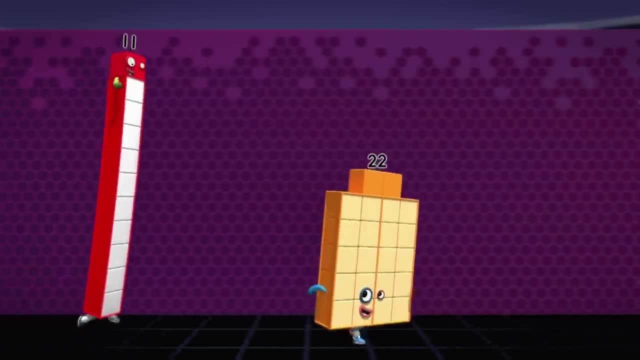 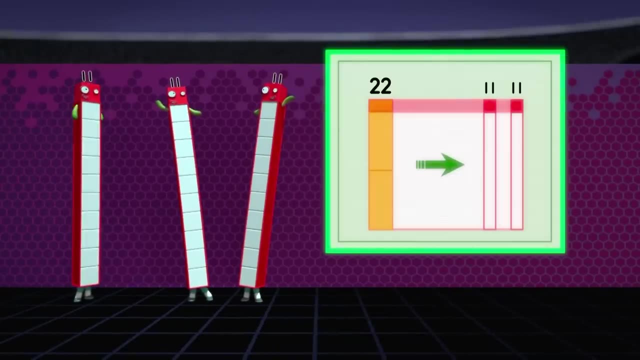 4, and 6. Oh 11 has already found 22.. Team of 11s: She tagged, She scored. Yay, Smaller numbers starting to Oh 10 is running. Big numbers, Big numbers. 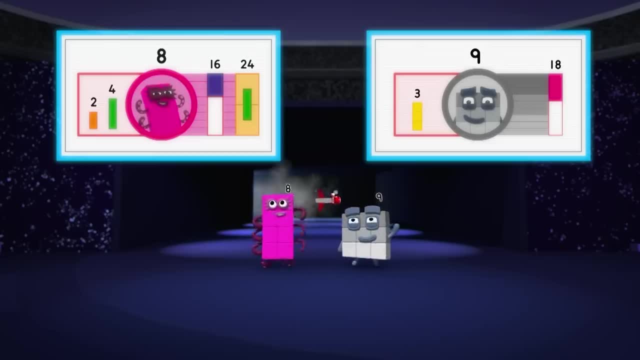 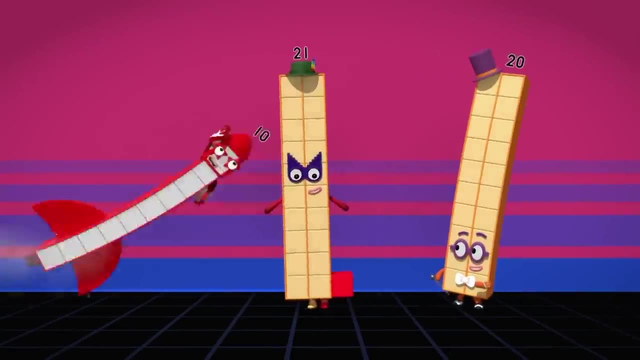 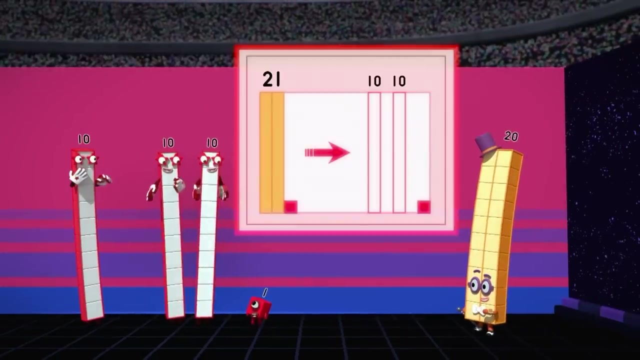 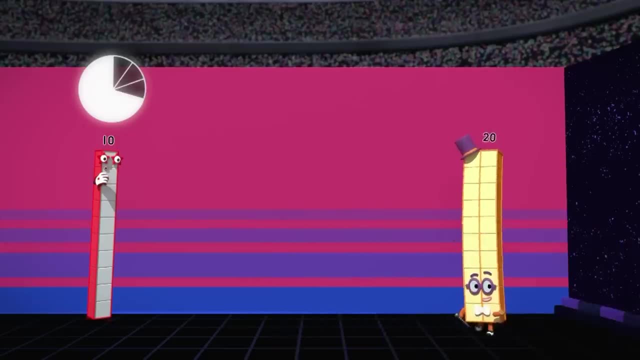 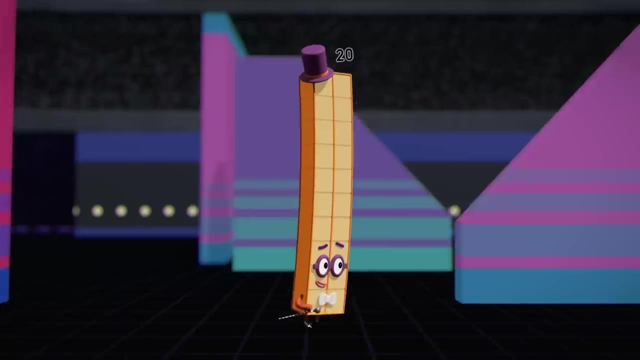 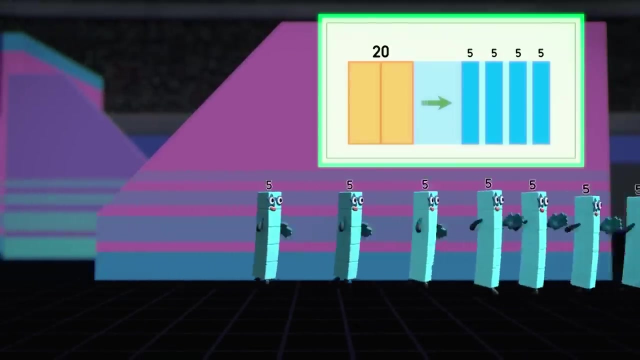 Oh no, He is't. Where did 5 come from? Team of fives, Team of fives. The fives off to a fantastic start there. They only need 15 to complete the set. Hush hush. 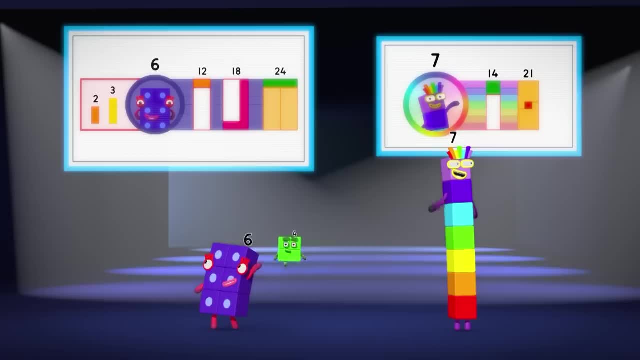 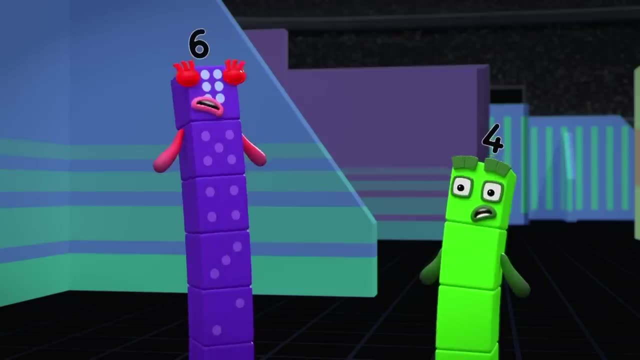 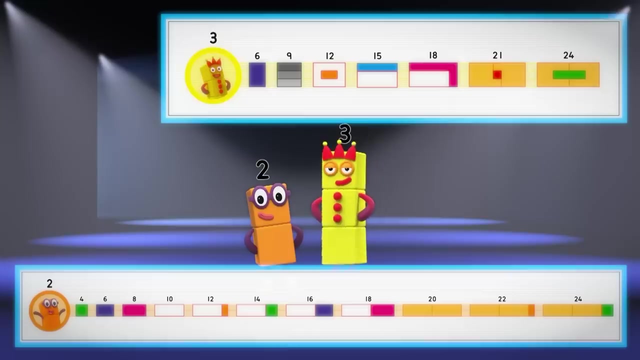 And if five is here, six and seven are already in. Lucky, lucky, lucky. And here comes four. But uh-oh, Look how many number blocks these two champions can catch, And with no one chasing them, you've got to fancy their chances. 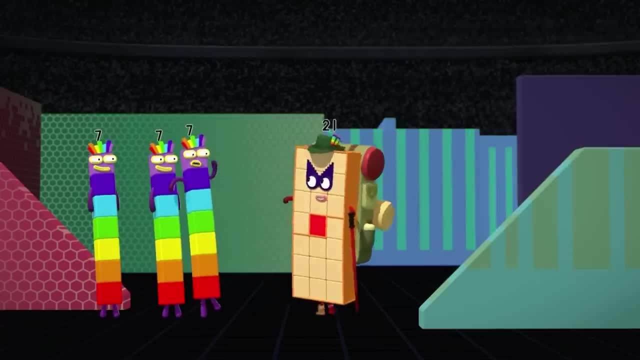 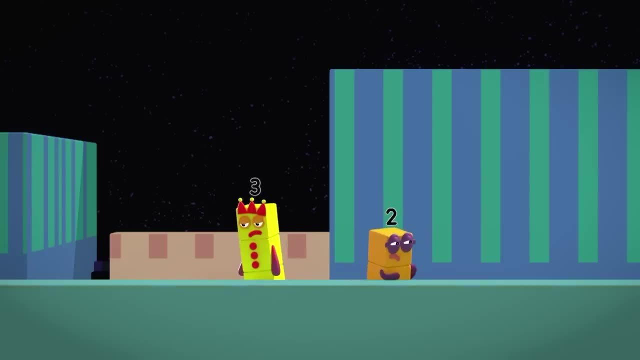 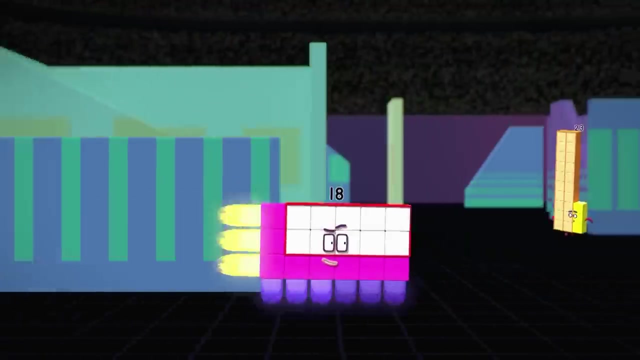 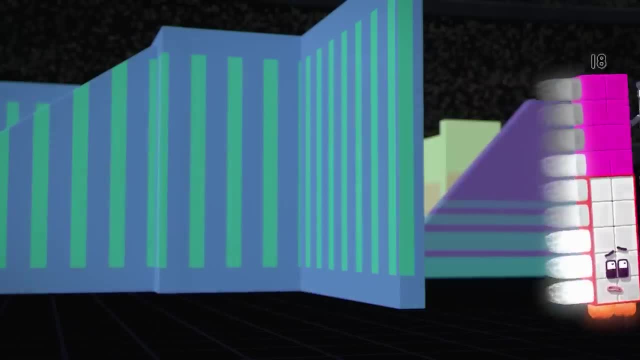 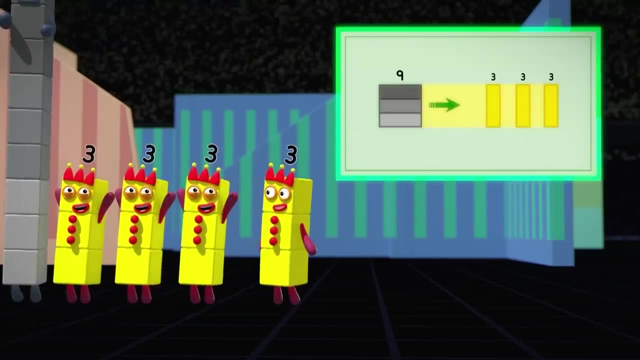 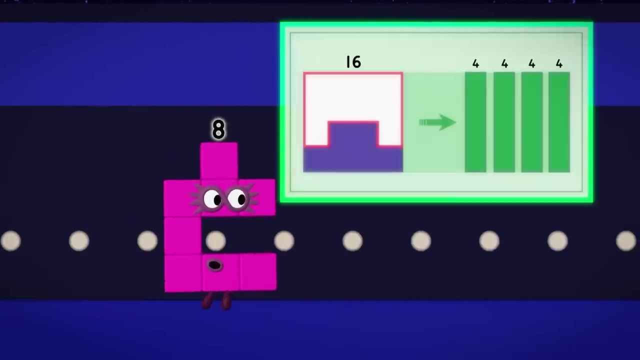 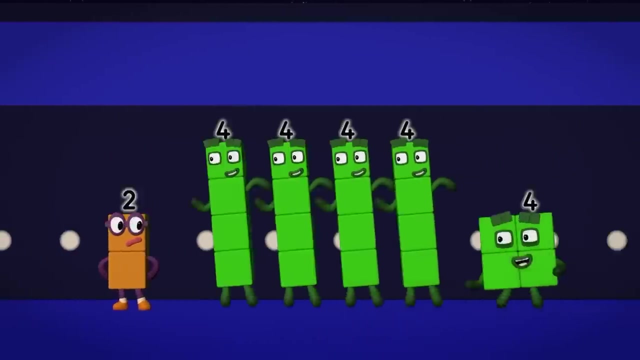 You can't catch me on a team of nines, Team of threes And sixteens in trouble, Octo-trouble. Team of fours Yikes Teams of twos. Twenty-four is still going strong. She could be the last rectangle standing. 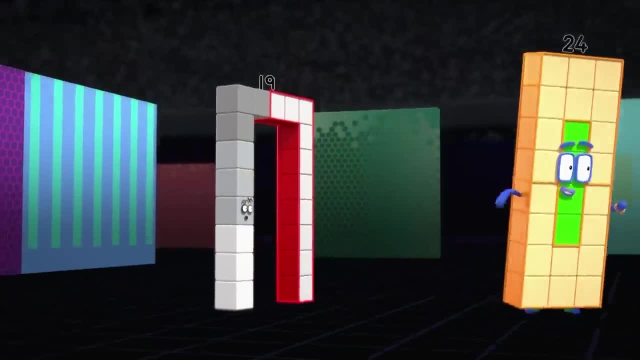 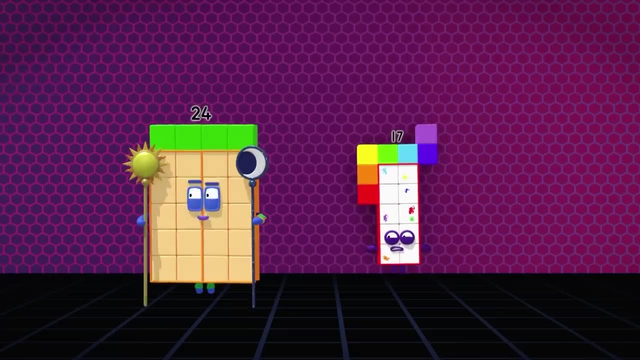 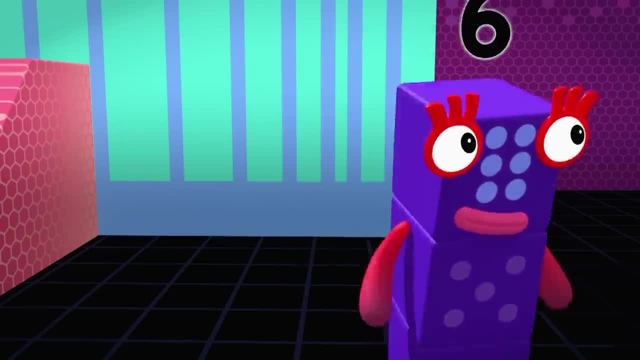 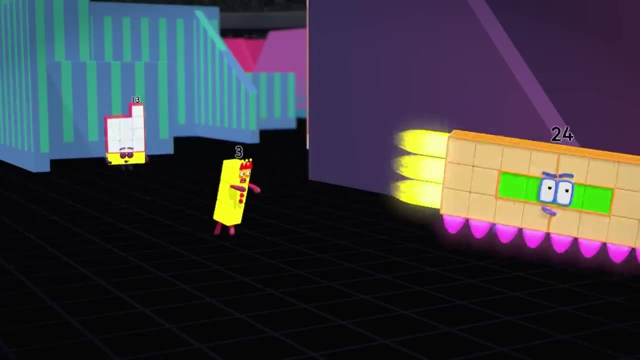 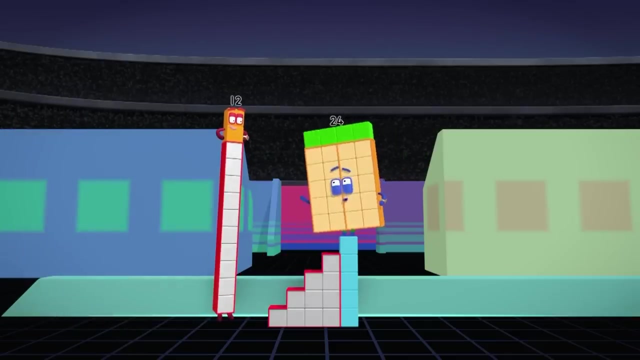 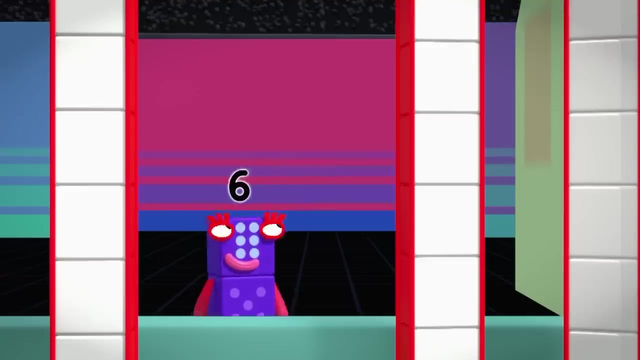 Ha, super-duper Right. Teams of twos. Hoo, Oh, Ooh, Hoo, Oh, well played, You've got me. Team of twelves. Hooray, Team of sixes, Team of sixes. 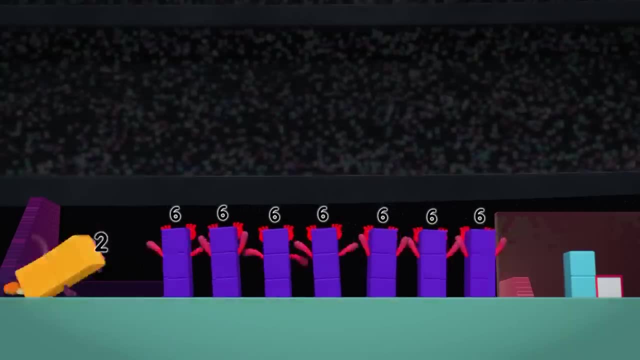 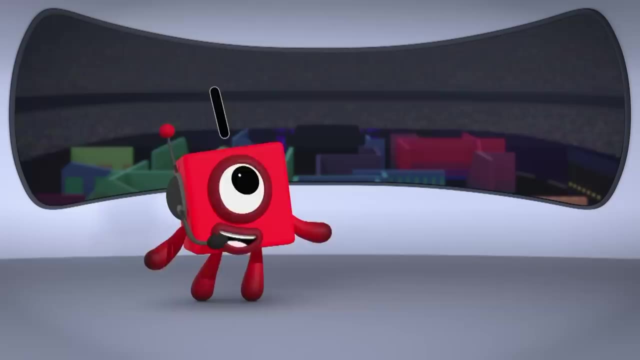 Hooray. Team of twos. Team of threes. Team of twos. Team of threes. Team of twos. Team of threes, Team of twos. That sound means it's last rectangle standing. Only one player remains who can be split into teams. 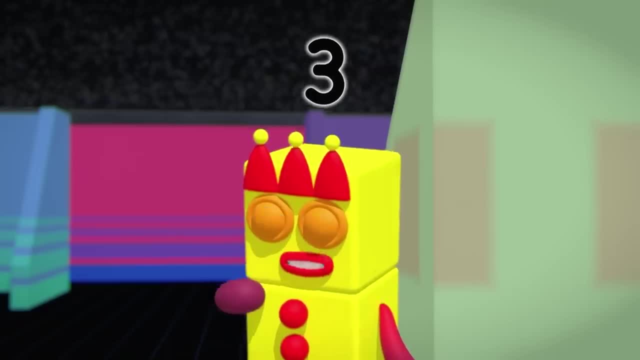 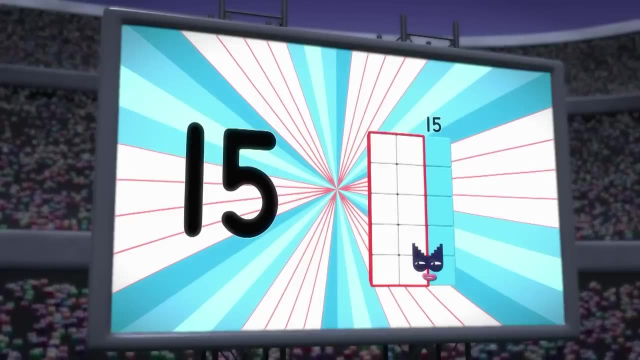 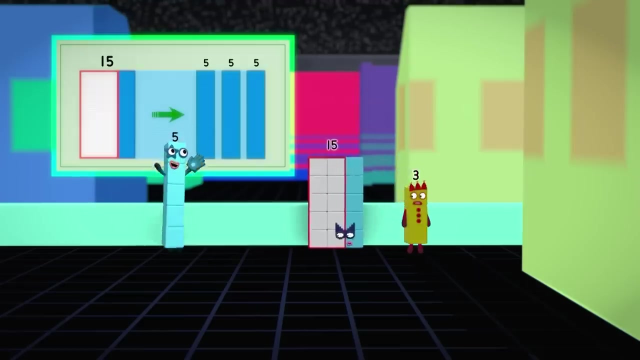 But who is it? Is there, Are you sure? there's a rectangle left, Hush, hush. Last rectangle standing is 15.. Aha, Team of fives, High five, Game over. And what a game it was. 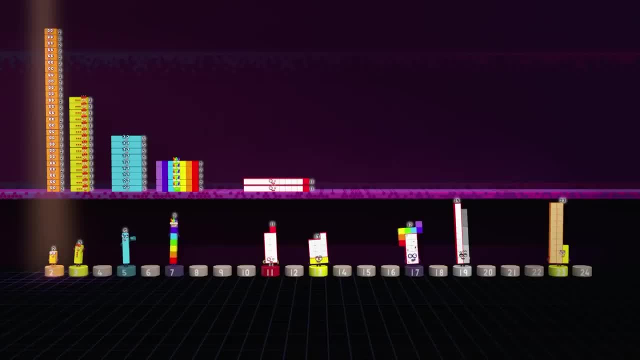 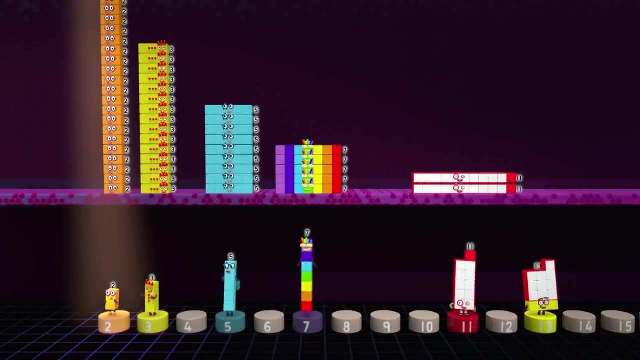 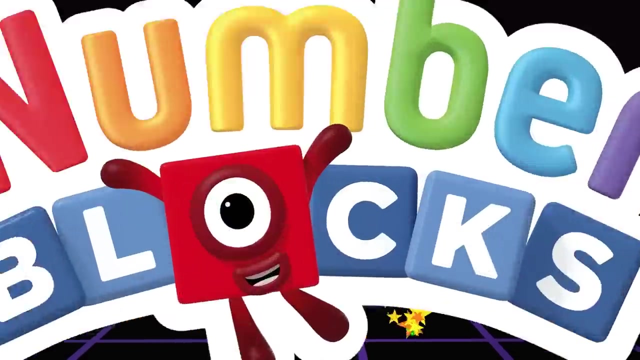 Let's find out who won. As the teams line up, only the not very rectangly number blocks are left And the winners are the twos. Yay, And that is Primetime Team Tag. That was a great day in the big city. 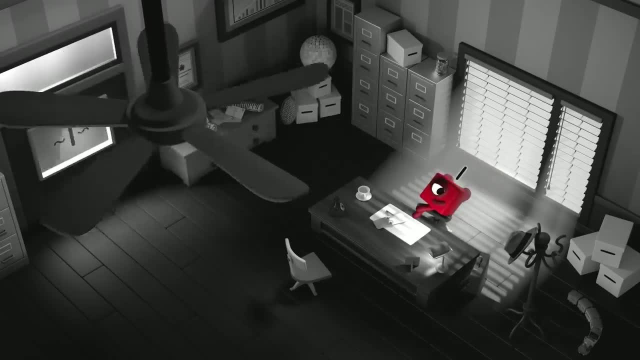 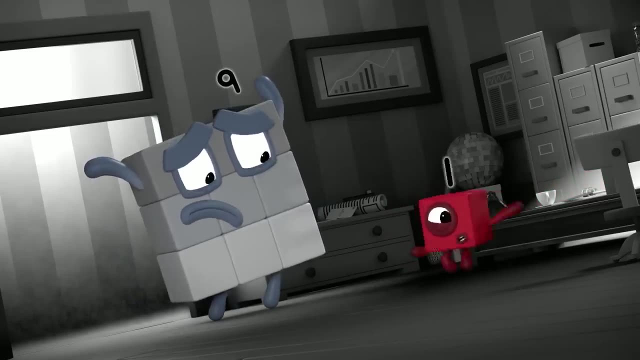 I was wondering where my next case would come from, when You've got to help me one. It's gone, Everything's gone. Slow down. Nine, Tell me what happened. I live in apartment nine on the ninth floor of numerical towers. 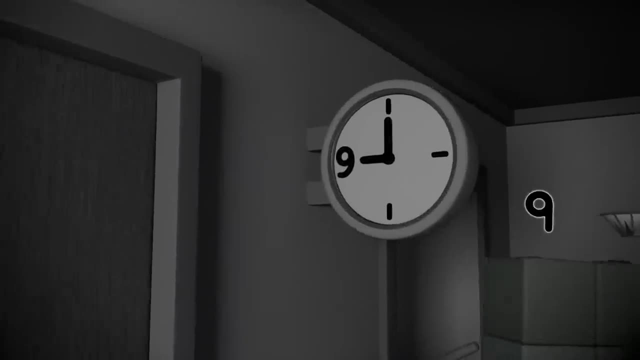 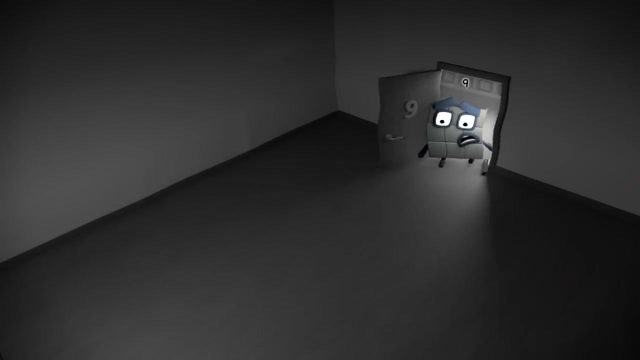 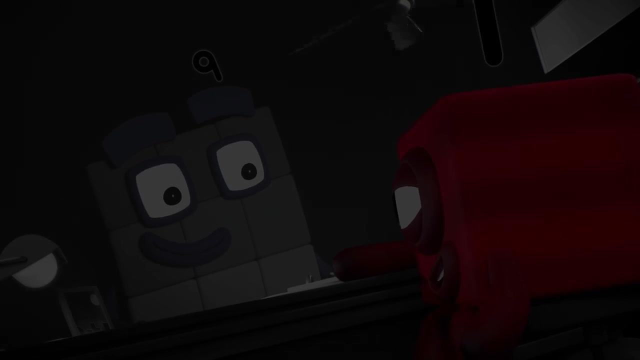 I left home this morning at nine o'clock to buy a newspaper. When I came back nine minutes later, the door was open. Everything was gone. A mystery indeed. I'll take the case. Let's look for clues. Did you notice anything strange or unusual when you got back? 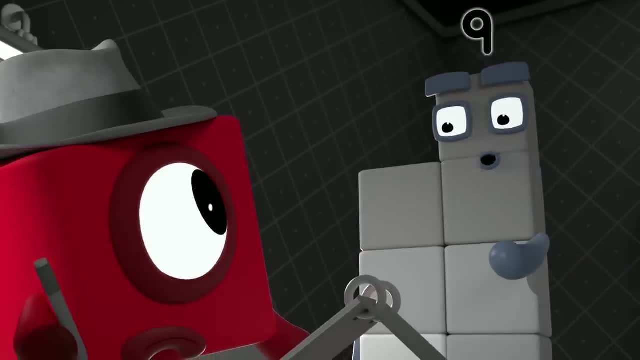 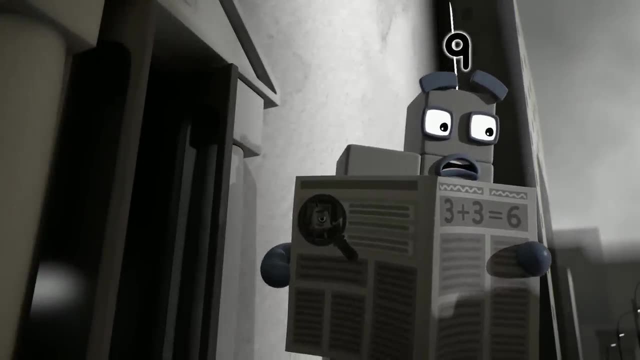 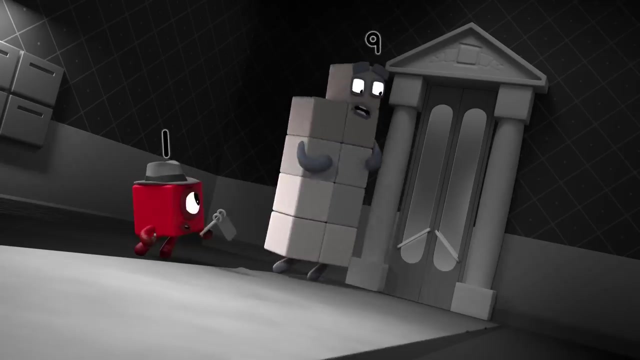 Uh, no, Nothing. Oh, there was one thing: A suspicious shadowy stranger in a coat and hat pushed past me and ran out of that door, But apart from that, nothing. Can you describe this stranger? They were as wide as the door, so two blocks wide, with a flat head. 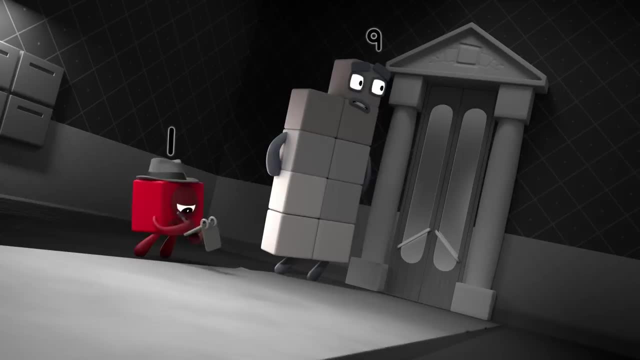 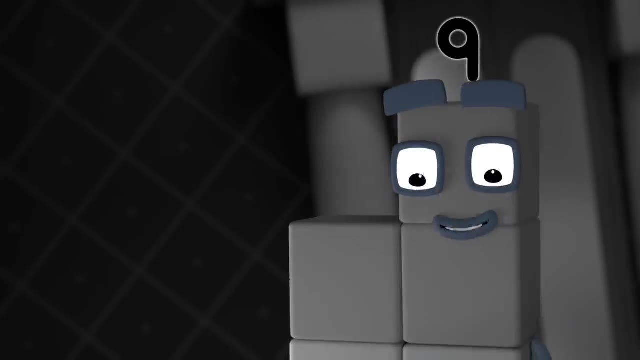 Clue one: Flat head when standing two blocks wide. Anything else I could see over their head when we were both two blocks wide, so they must have been smaller than me. Clue two: Smaller than nine. Look, Hat, Coat. 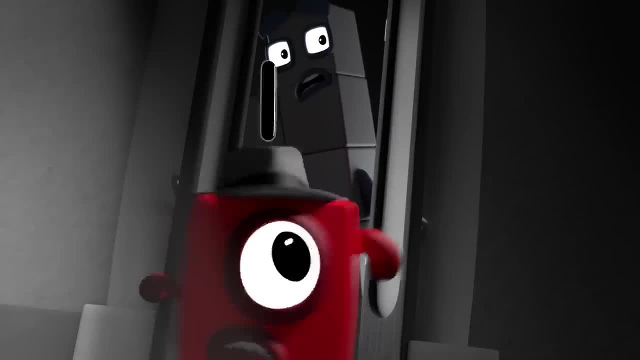 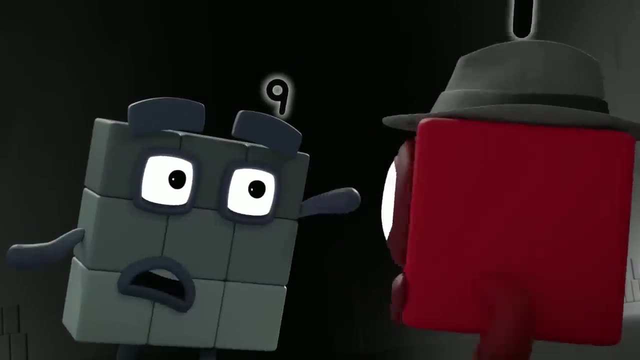 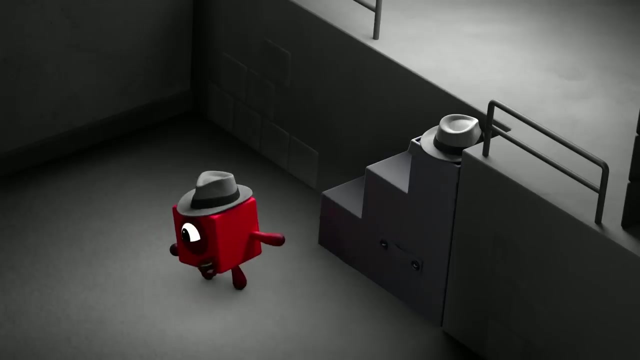 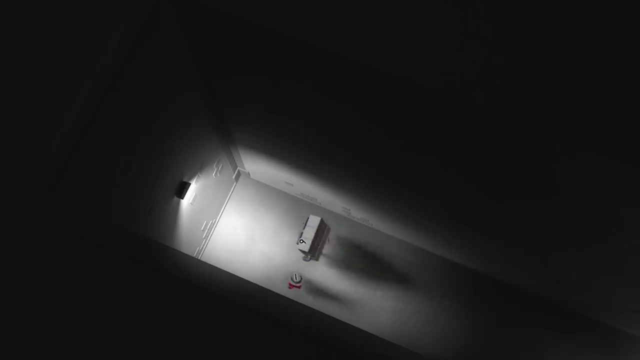 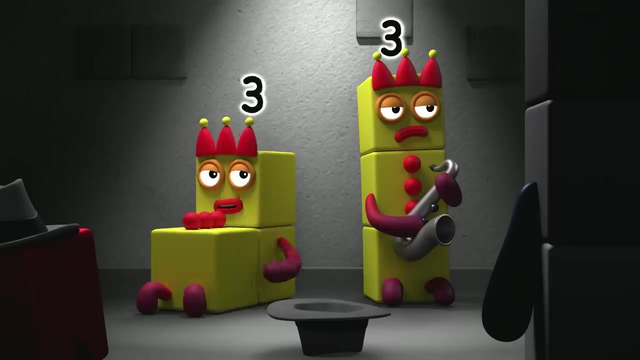 It's them. After them, quick There On the steps. The hat. These aren't steps, It's. Did either of you see a suspicious step-shaped figure in a coat and hat? Sorry, friend, No one else down here. 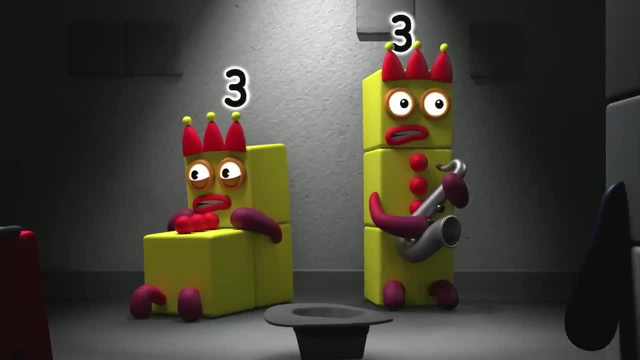 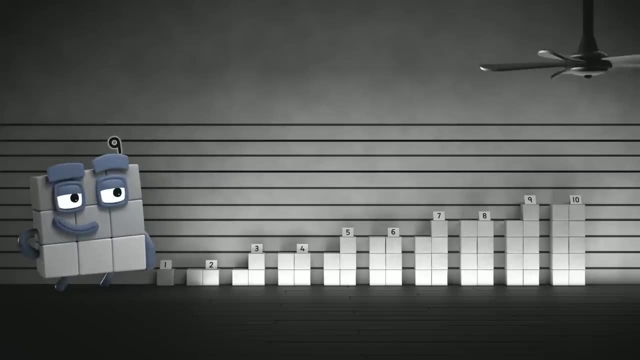 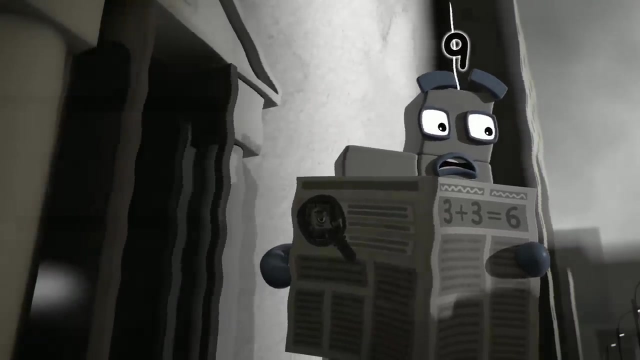 Just us. Something didn't add up, Ordid it. Let's look at what we know. Clue one: The suspect had a flat head when standing two blocks wide, So it can't have been three, five, seven or nine.